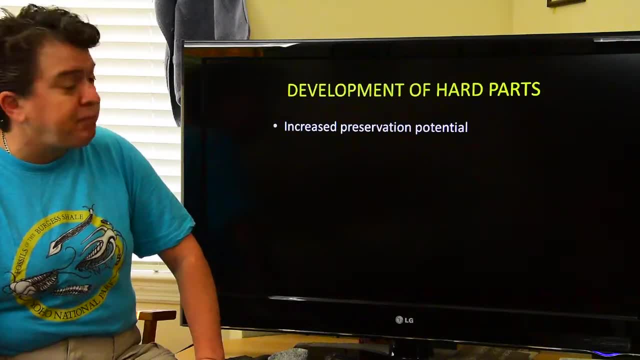 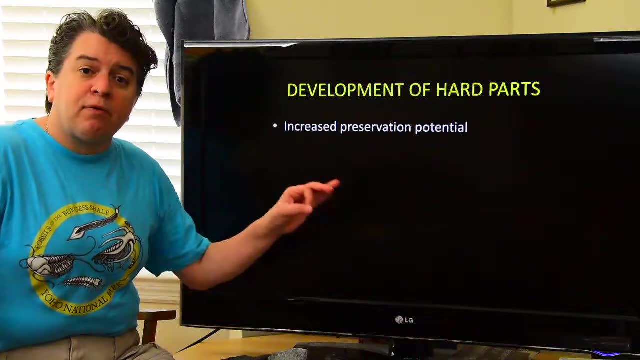 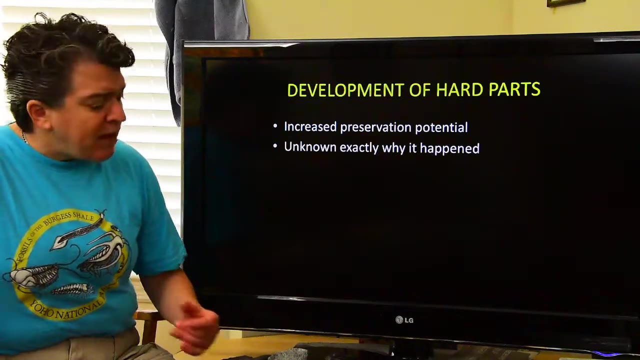 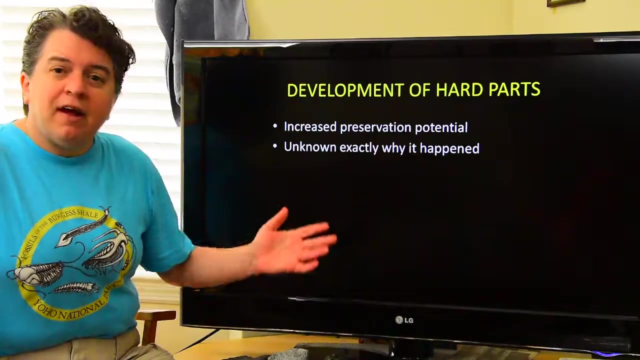 a major development of hard parts- shells and things like that- And this important development increases the preservation potential of fossils. So we start seeing more life forms because they are better preserved, And the thing about this major advance in life, we don't exactly. 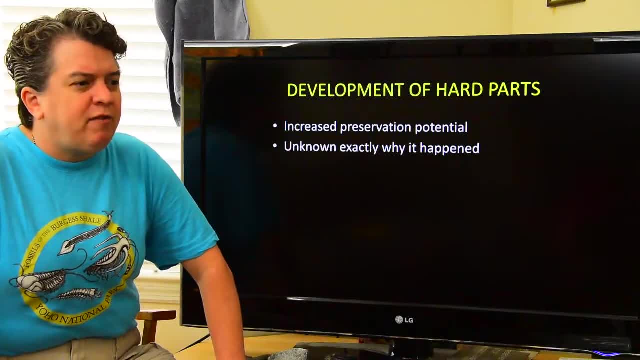 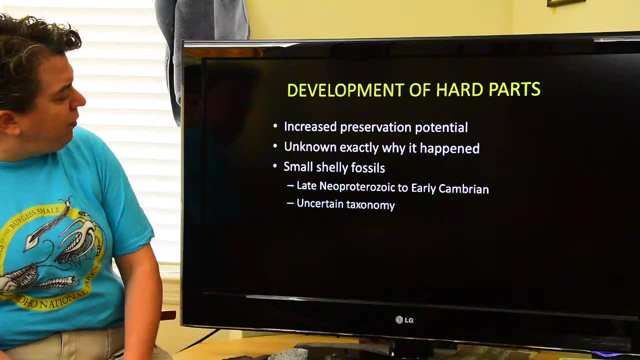 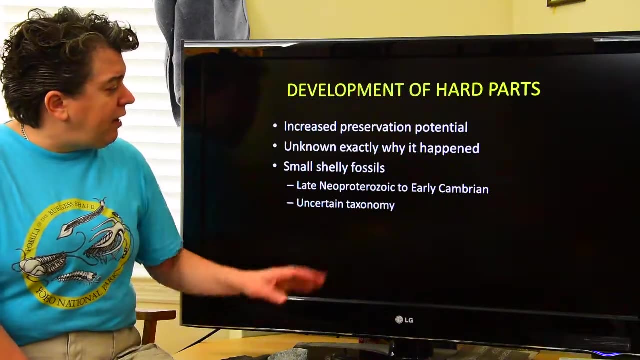 know why it happened. We are not sure why life began developing hard parts, but it happened, And some of the earliest life forms we see with these are these things that we call small shelly fossils. That is seriously the name we have for them- And they show up in the late Neoproterozoic. 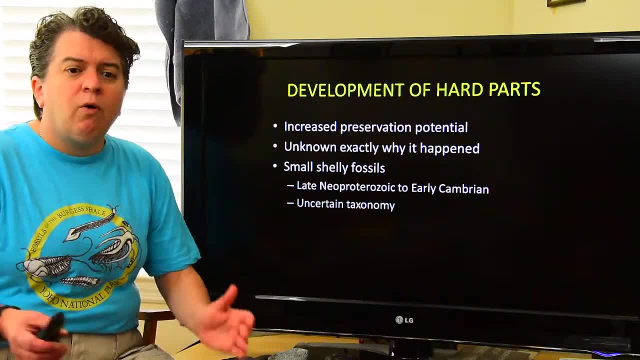 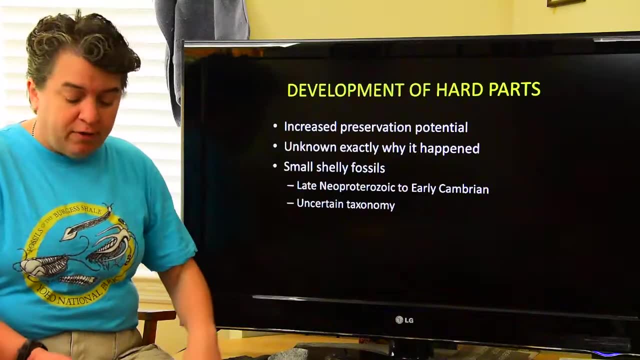 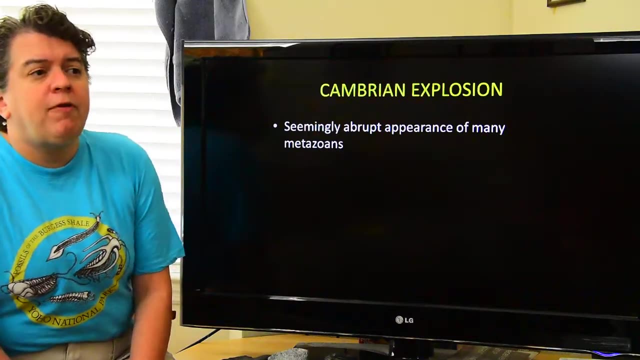 and exist into the early Cambrian. We don't exactly know what life they are related to, what life forms, so we don't know the exact taxonomy, But they are there and they are some of the early things that developed hard parts And in the Cambrian. one thing very noticeable also is we get a lot of metazoans, Remember. 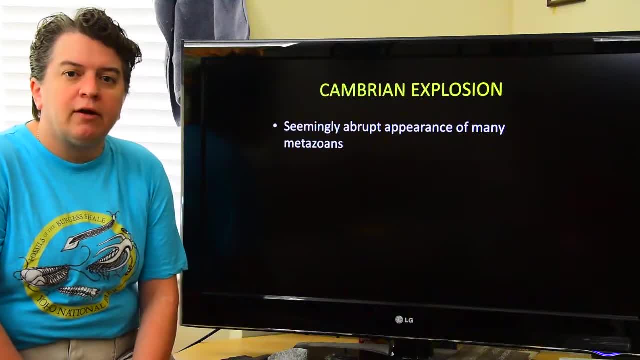 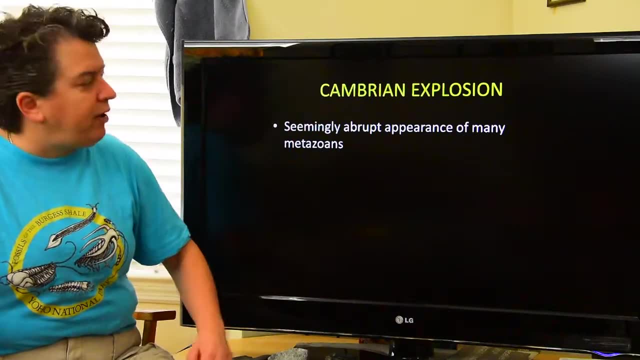 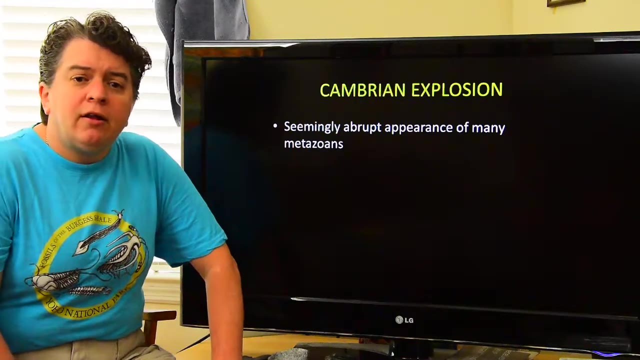 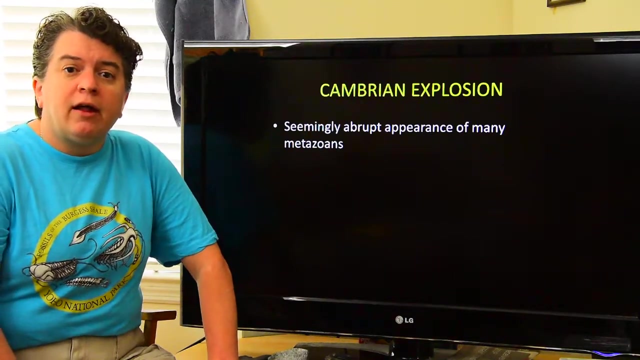 those larger multicellular organisms. And this appearance of all these larger multicellular organisms is called the Cambrian explosion, And I wrote that it is a seemingly abrupt appearance because for a long time we did not know about some of the older metazoans that inhabited the Neoproterozoic, like those Ediacaran fauna organisms. But basically, in 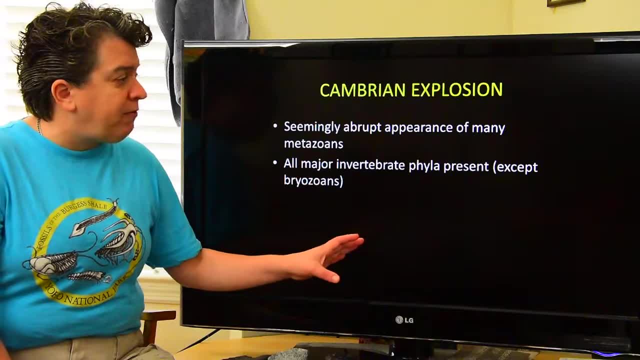 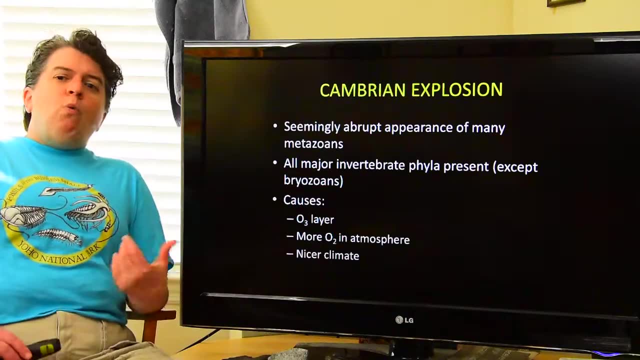 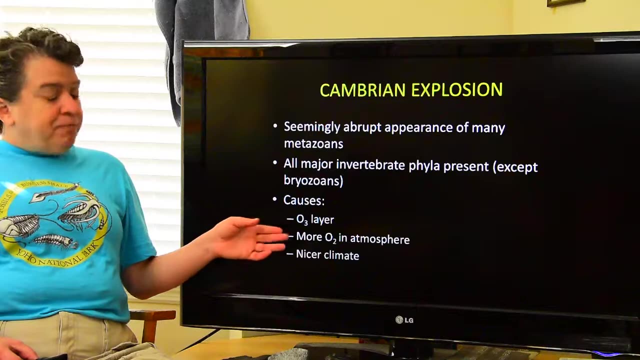 the Cambrian explosion, we see all major invertebrate phyla except the bryozoans. They come along a little bit later. And why did the Cambrian explosion happen when it did? Well, there is a few possible causes. There is more ozone in the atmosphere, which does offer a measure of protection from 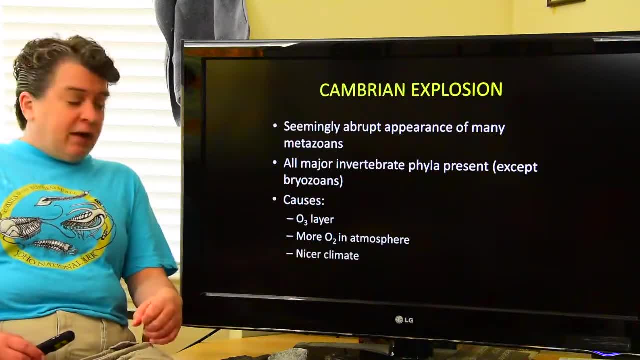 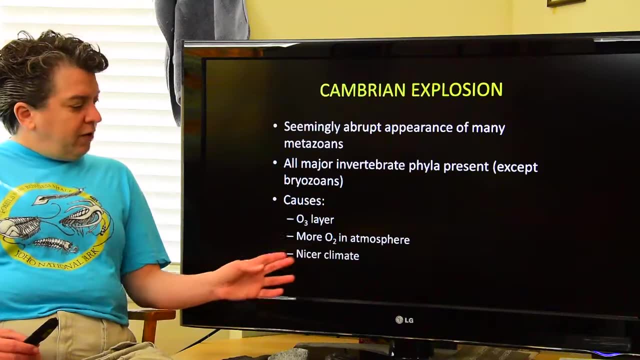 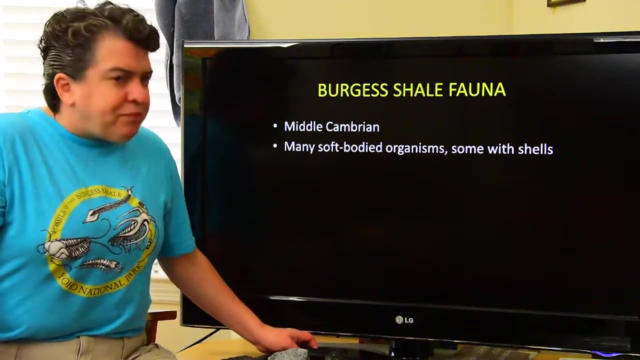 UV radiation. There is more oxygen in the atmosphere for these organisms- And remember we just came out of some snowball earth episodes- And so it could also be that we just have a nicer climate at this time And some of the important organisms that we see at this time belong to what is called 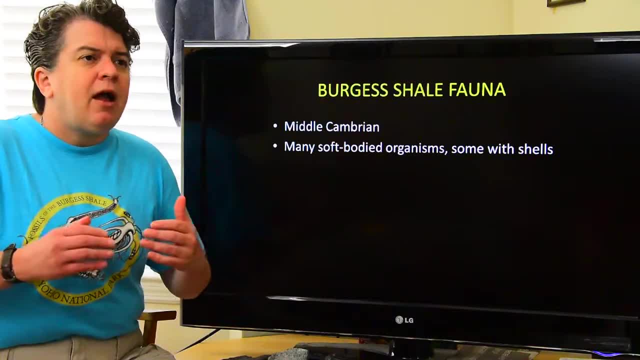 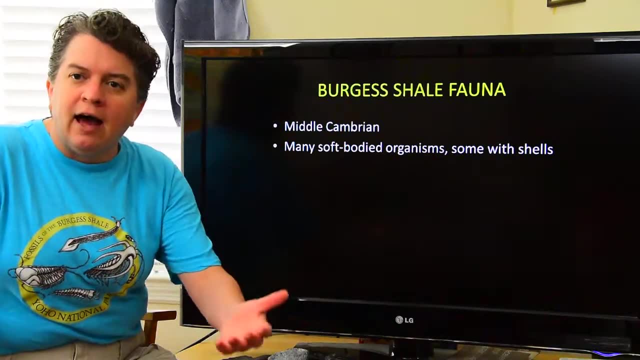 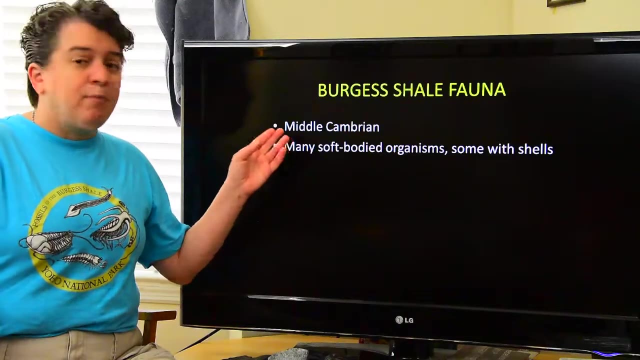 the Burgess shale fauna. Every now and then in geology we have these just really important groups of animals like that Ediacaran fauna of the Precambrian. The Burgess shale fauna is important. It is in the middle Cambrian. It includes a lot. 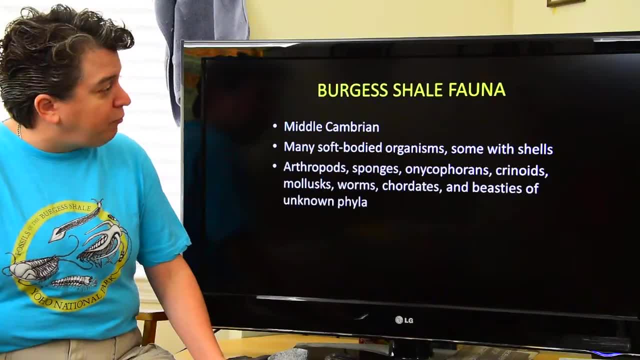 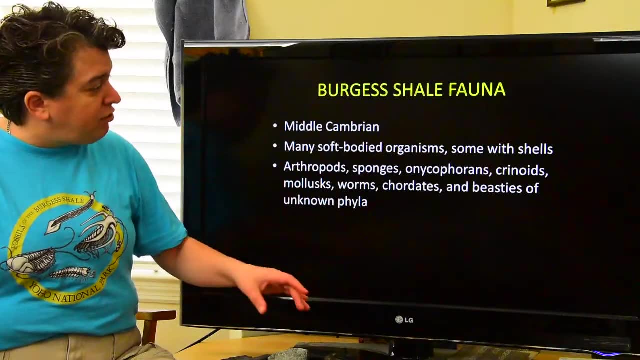 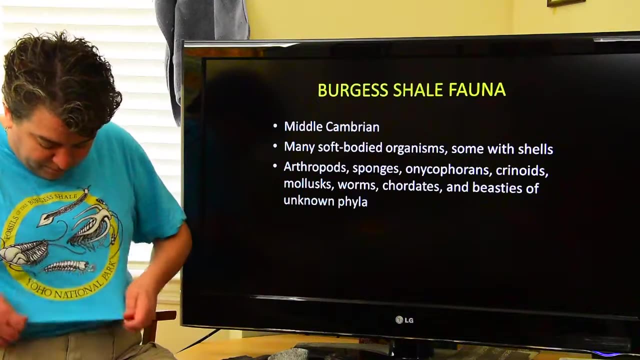 of soft body organisms, but it does also include some with shells, And we have all kinds of different organisms, Arthropods and sponges, These weird things, Onychophorans, crinoids, mollusks, worms, chordates and beasties of unknown phyla. Some of them are shown here. 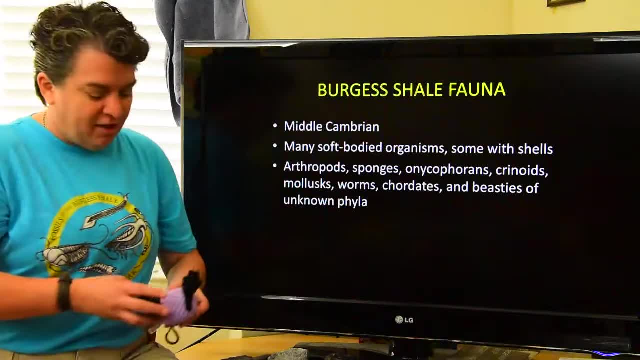 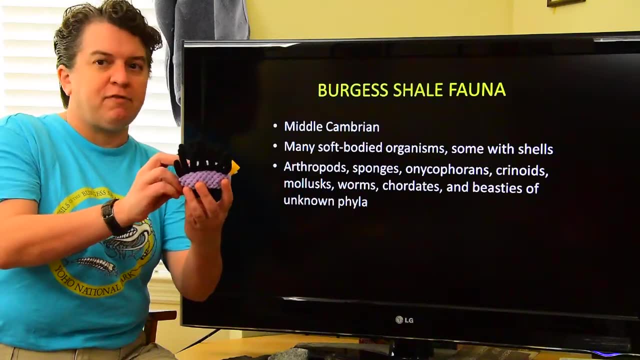 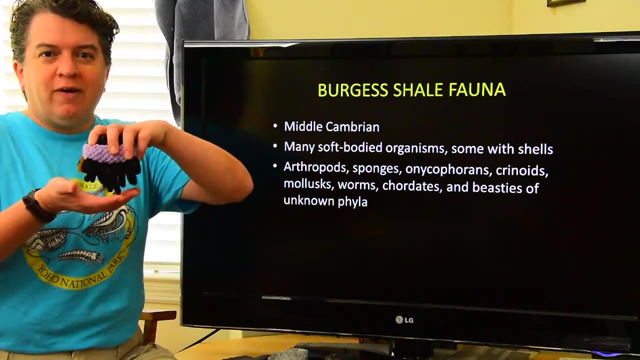 on my nice t-shirt And some of the interesting ones, Or like this guy. This is called Wewaxia, And when people originally found this fossil of Wewaxia, they actually thought that it walked on the ground like this, But ended. 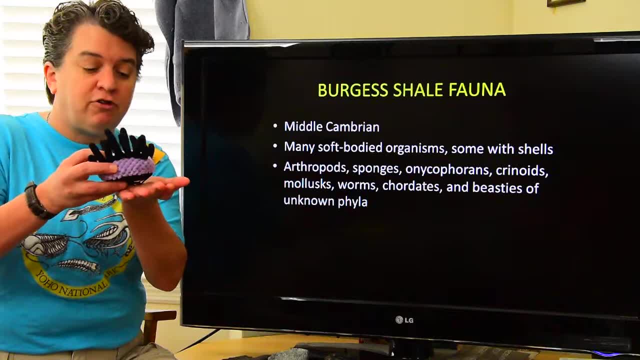 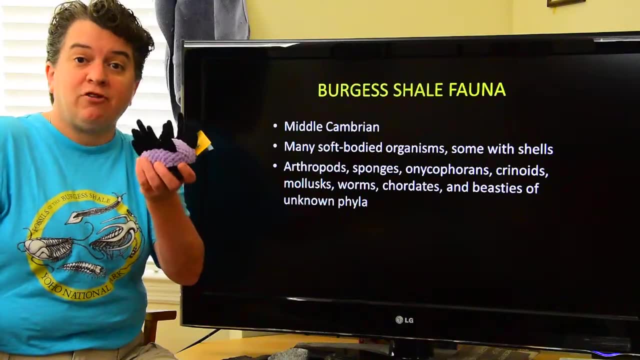 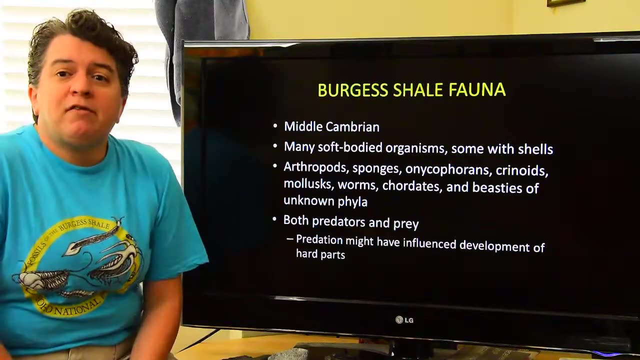 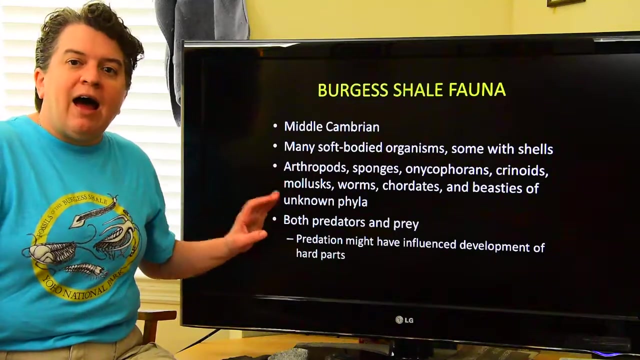 up that it actually moved. It lived in the ocean And it basically would walk along the seafloor like this, And these were probably for some sort of protection. And what makes this Burgess shale fauna so interesting to paleontologists is we actually see both. 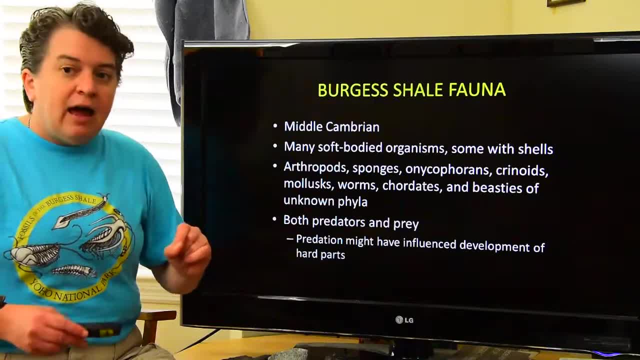 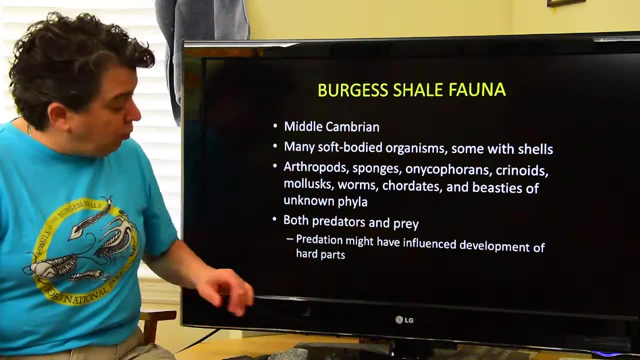 predators and prey animals And it is thought that another one of those reasons hard parts developed or the weird little spines on that Wewaxia and stuff, is that predation might have influenced the development of hard parts. Because it is thought that the hard parts 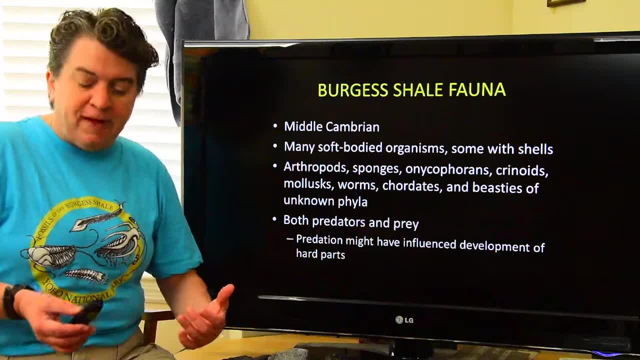 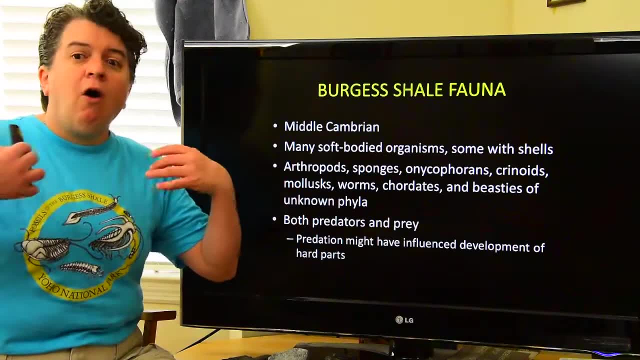 might have influenced the development of hard parts, Because it is thought that predation might have influenced the development of hard parts, Because it is thought that predation it became something defensive for organisms to have. So the Burgess shale fauna is important to us because, like I said, we have all kinds of different animals And we have both predators. 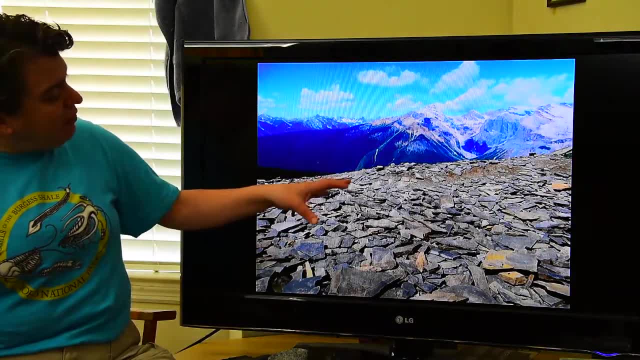 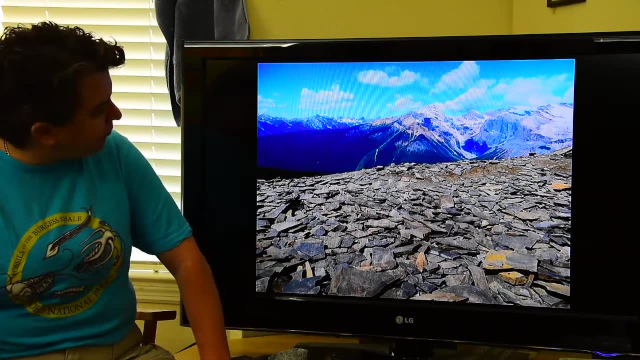 and prey, And we are seeing that interaction between those. This is the Burgess shale. This is off in Canada in a place called Yoho National Park, And there we see an artist's rendition of what Burgess shale fauna looks like. This is the Burgess shale fauna. This: 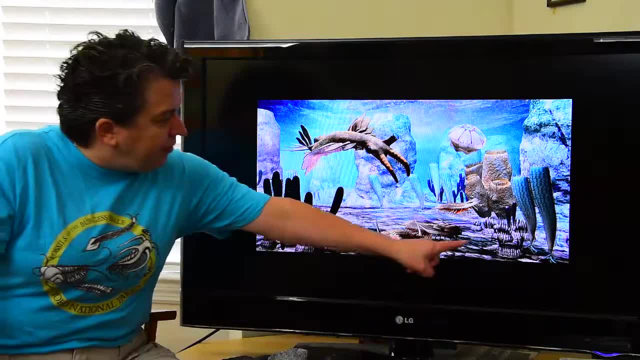 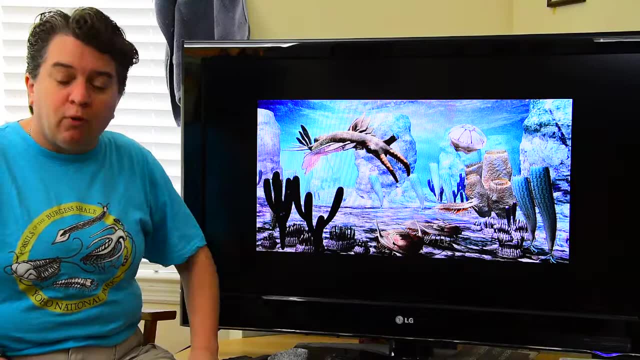 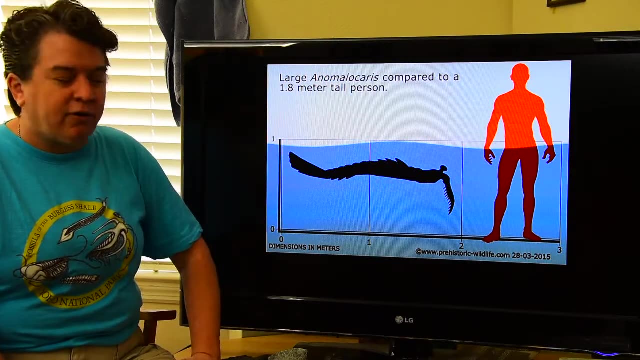 is what the Burgess shale fauna would have looked like. Here we have some Wewaxias I was showing you and some Trilobites, And there is this very important predator in there, That guys animalocaris, and you can see how large that predator could get compared to. 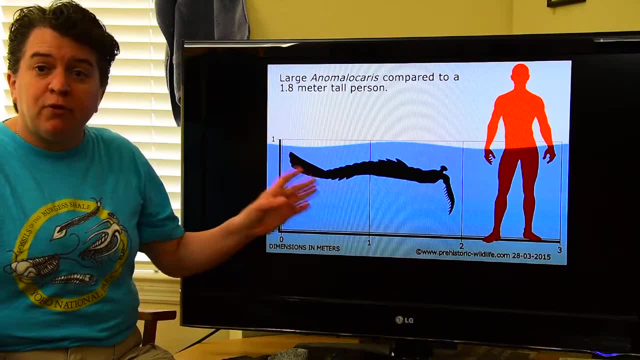 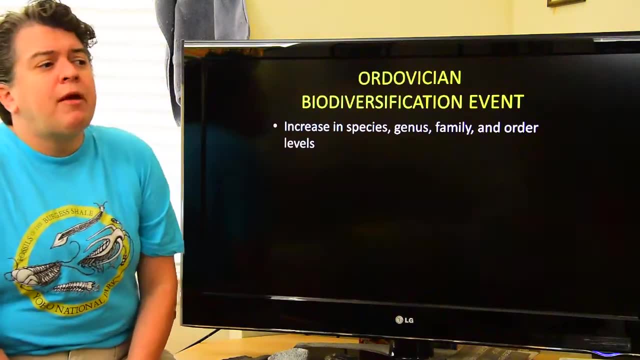 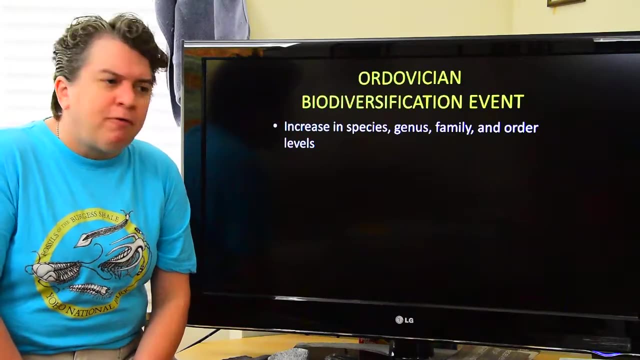 a six foot person there. So this is a major predator of that Cambrian time period. Now, Now, when we leave the Cambrian and enter the Ordovician, life really diversifies And we call this the Ordovician Biodiversification Event. 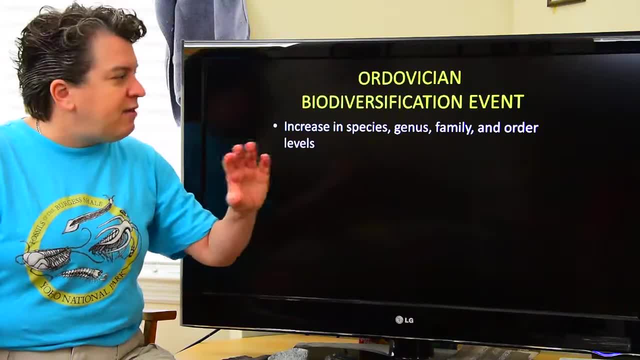 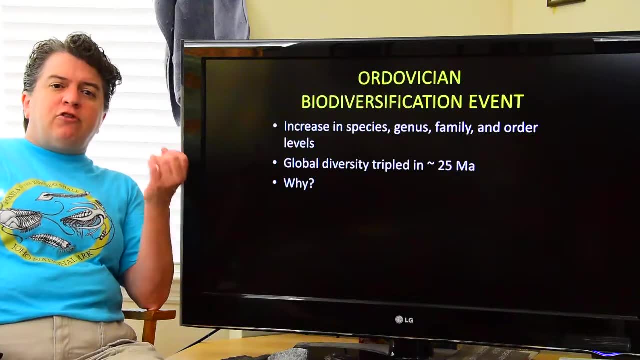 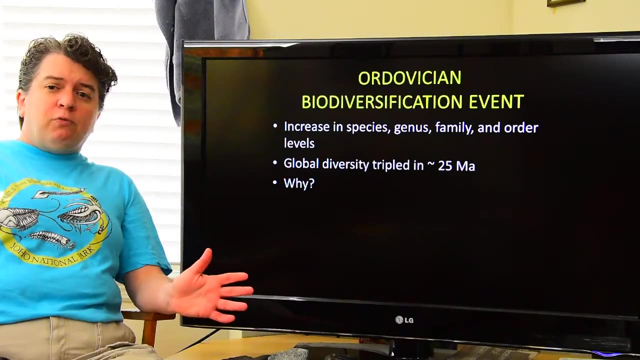 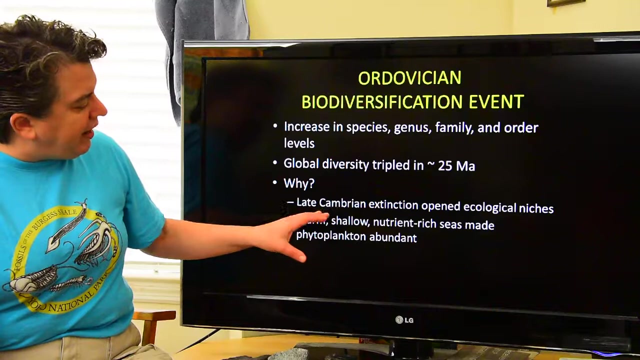 And we see a major increase in species, genus, family and order levels, And, in fact, global diversity tripled in about 25 million years during this event, which leaves paleontologists wondering why. Why would that happen? Well, there was a small extinction event in the late Cambrian. 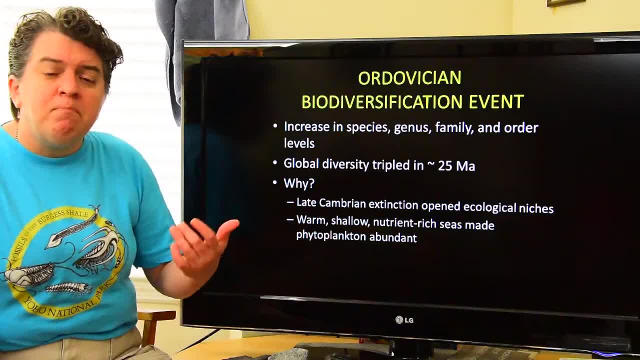 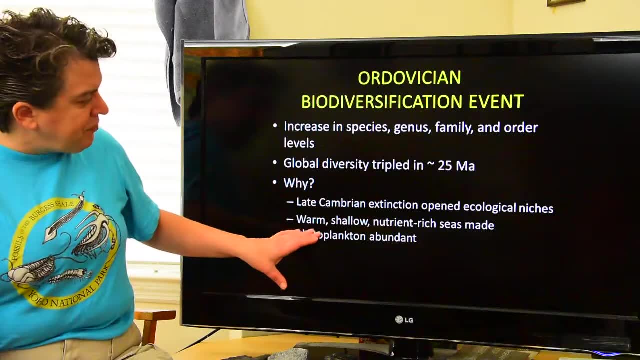 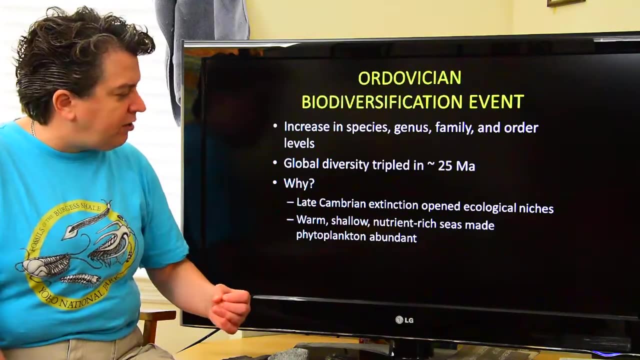 And that extinction event might have opened ecological niches for new organisms to diversify and then occupy. But then remember, in the Ordovician we had these warm, shallow epicontinental seas. They're very nudist, They're nutrient-rich. 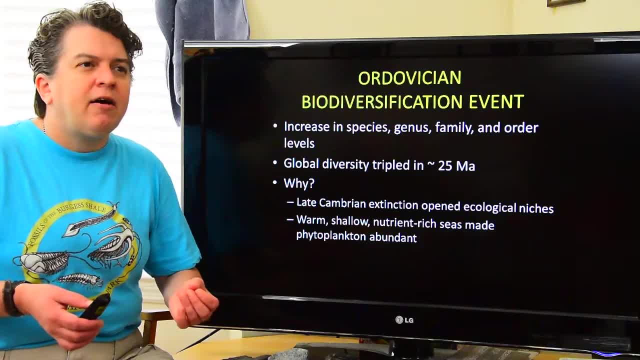 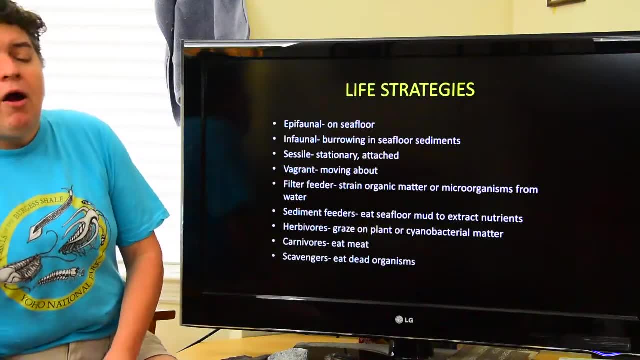 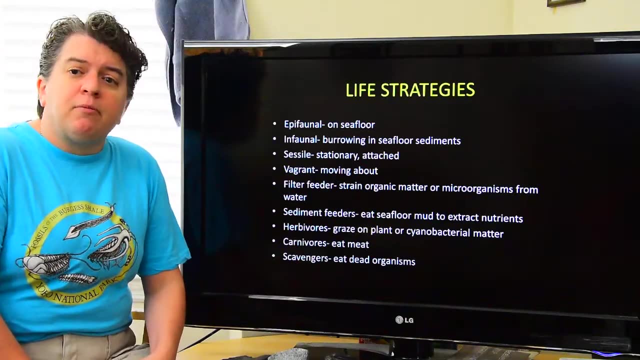 Phytoplankton's abundant, So it just might have been kind of the perfect environment for this diversification to occur. Now, as I go through different life forms of the Paleozoic, I'm going to be using some terms to describe their life strategies. 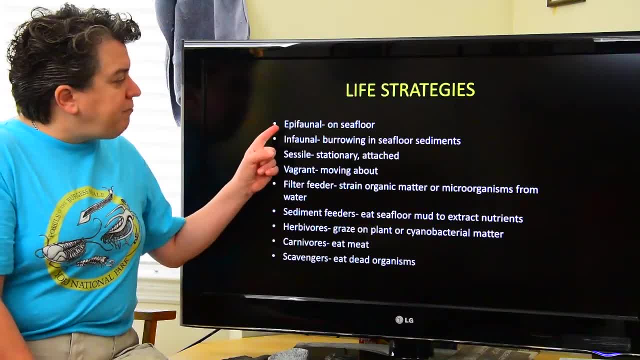 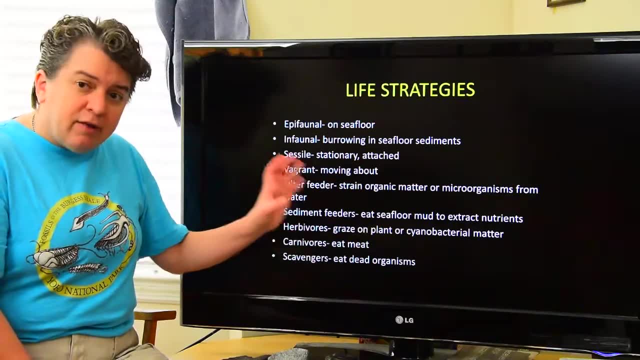 So these are some terms I want you guys to remember, And some of them we already went over Back when I first introduced fossils and fossilization. But let's just have a nice little review then. So we have epiphaunal means- it's on the seafloor. 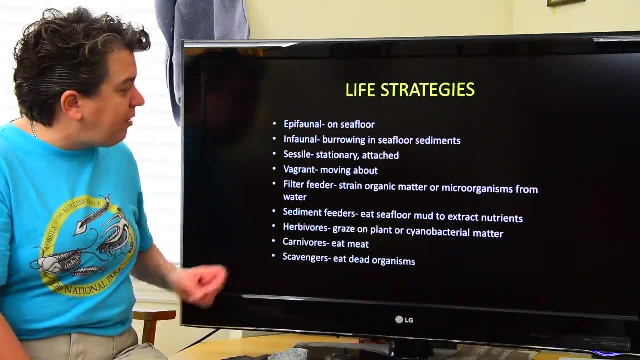 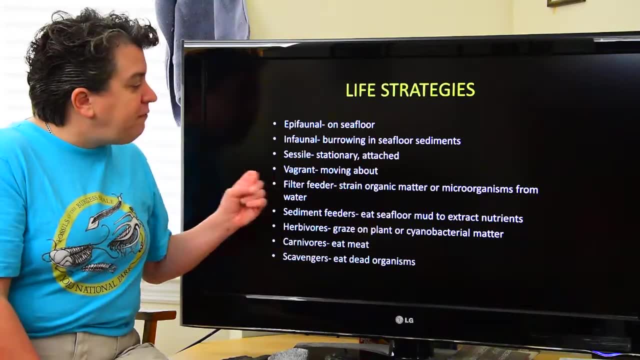 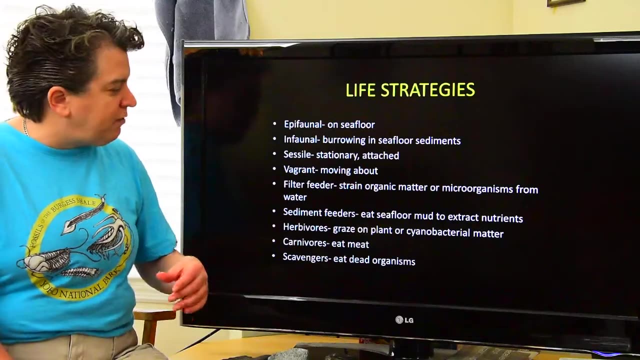 In-phaunal is burrowing into the seafloor sediments. Sessile means that it is stationary, It's attached to something It doesn't move around. Vagrant means it moves around. Filter feeders strain organic matter or microorganisms out of water. 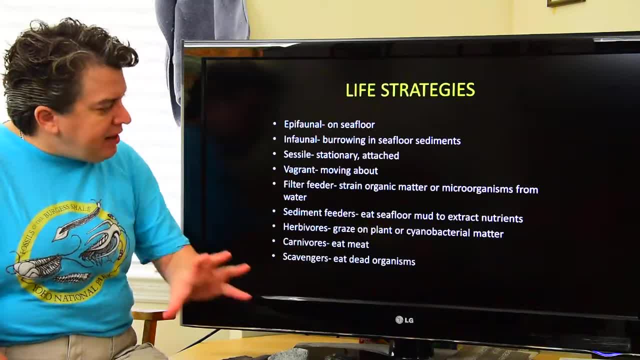 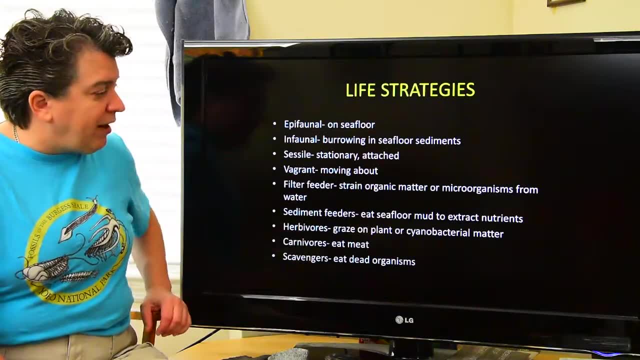 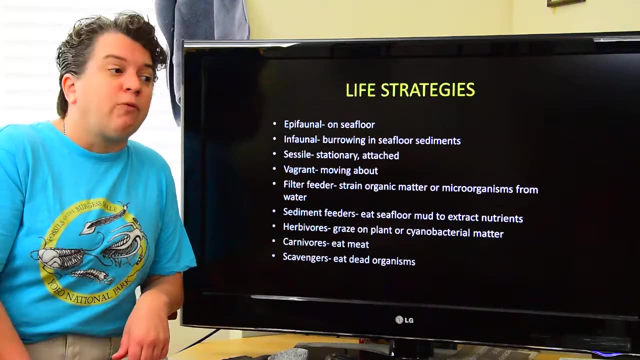 Sediment feeders actually eat muds on the seafloor and basically extract the nutrients from that. Herbivores graze on plants, or cyanobacteria Carnivores are meat eaters, And then scavengers go after things that are already dead. 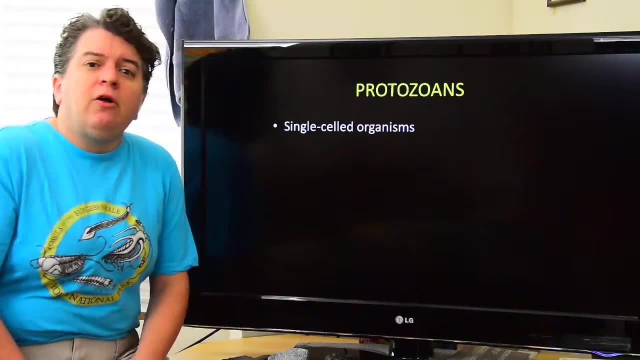 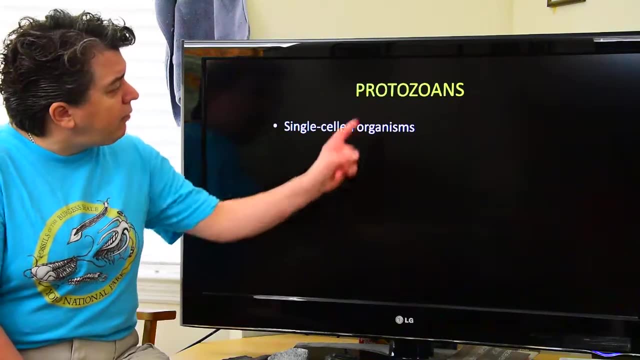 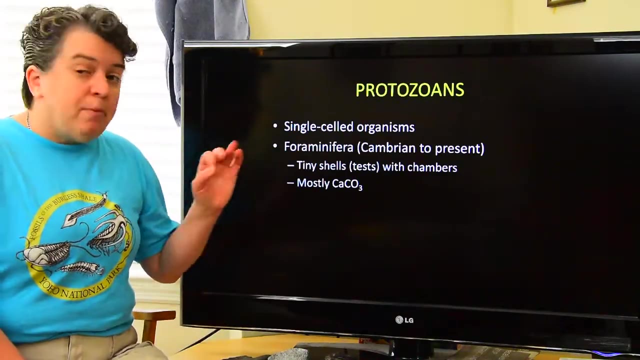 So let's then take a look at life and different life forms that existed in the Paleozoic. We're going to start with our protein Protozoans. Protozoans are single-celled organisms, And a major group of these are the foraminifera. 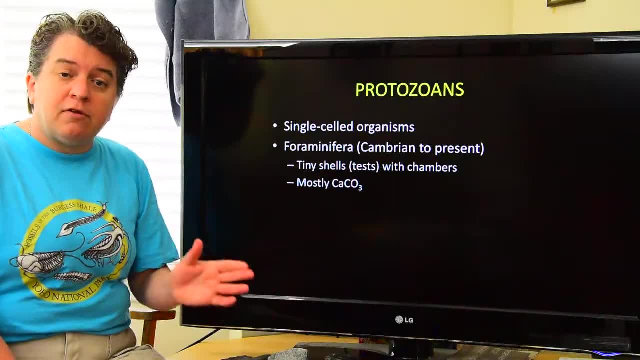 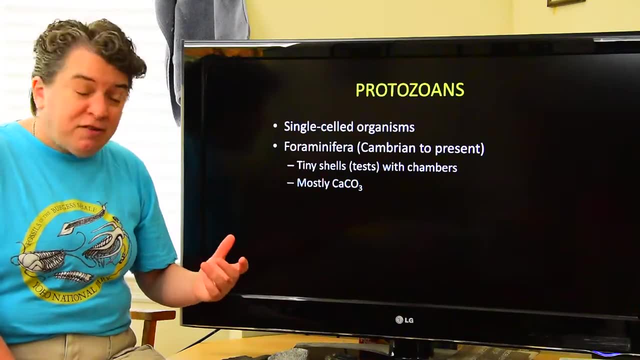 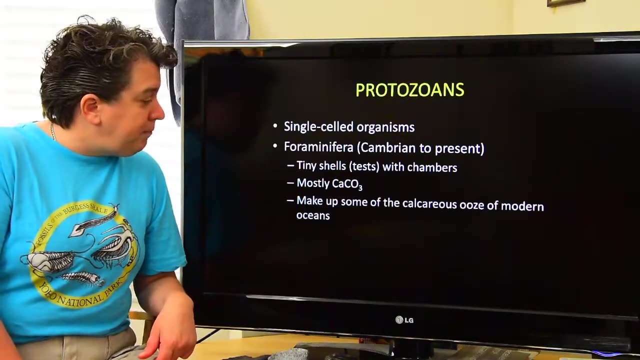 They show up in the Cambrian and they still exist today, And these are really, really tiny shells, which paleontologists call tests, And they have little chambers inside of them. Most of these are made from calcium carbonate, And when we went over the calcareous, 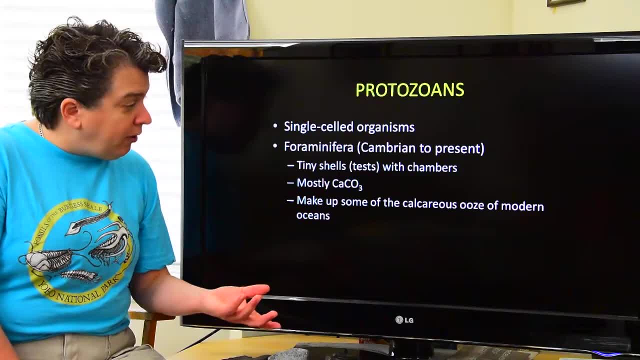 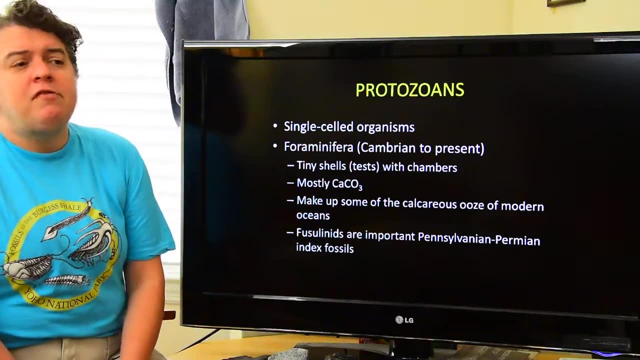 Calcareous, Calcareous, Calcareous ooze that accumulates on the seafloor, Remember that. Well, this makes up some of that calcareous ooze. Now, in these protozoans, these foraminifera, which we often call forams for short, there's 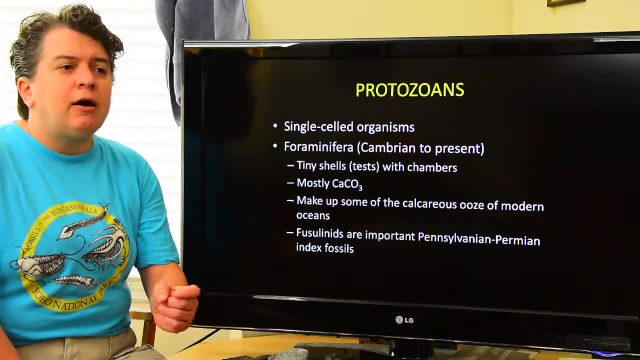 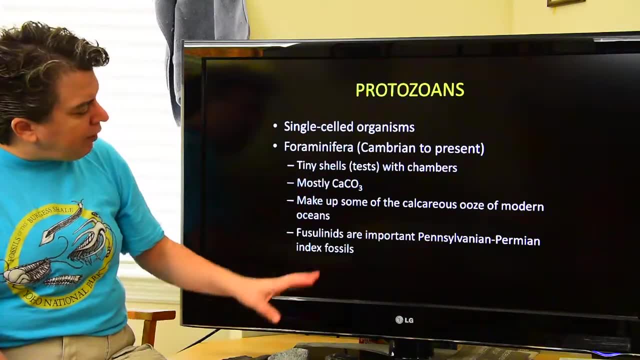 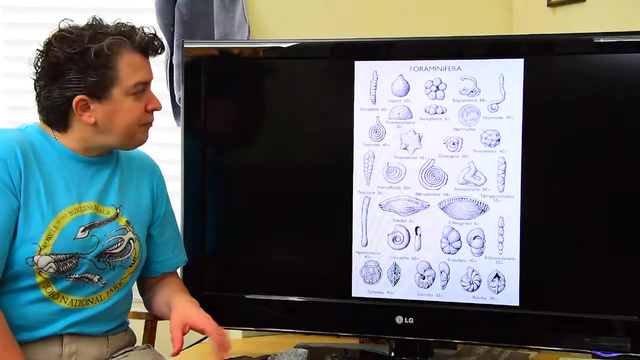 a group called fusulinids. You saw that in the fossil lab. Those were some of those little rice-shaped fossils. Well, they're an important index fossil In the late Paleozoic And here's an example of some of the different forams that you might have. 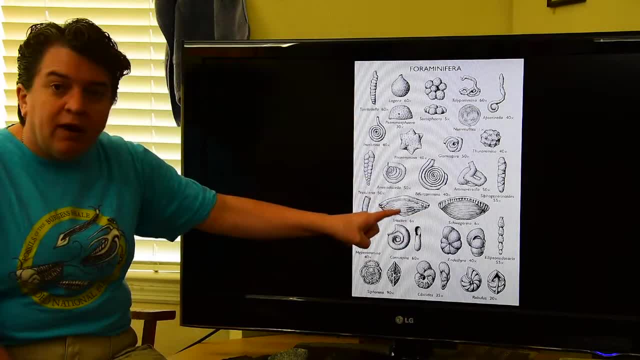 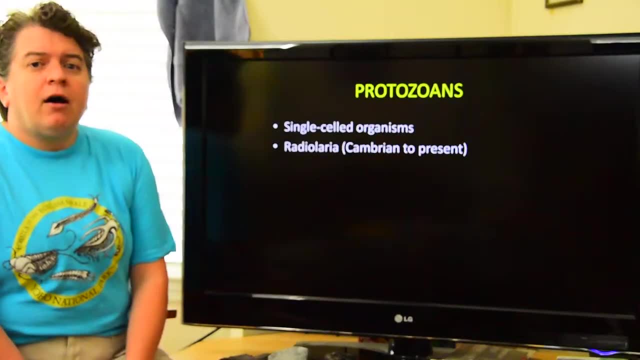 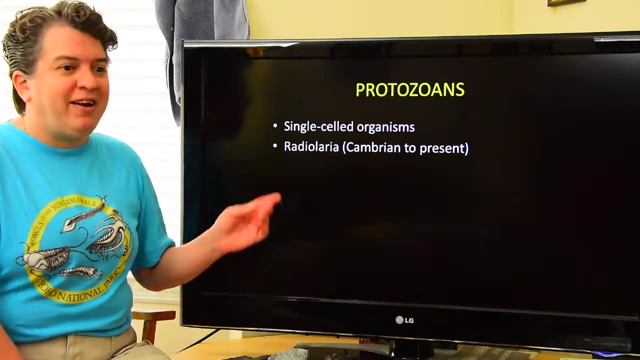 You guys saw this one- or maybe it was this one, the little grain of rice looking one in the fossil lab. But forams aren't the only single-celled organisms out there. We also have radiolarians, Radiolarians, Radiolarians. 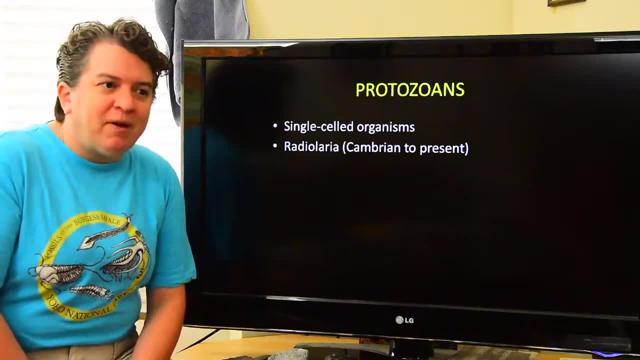 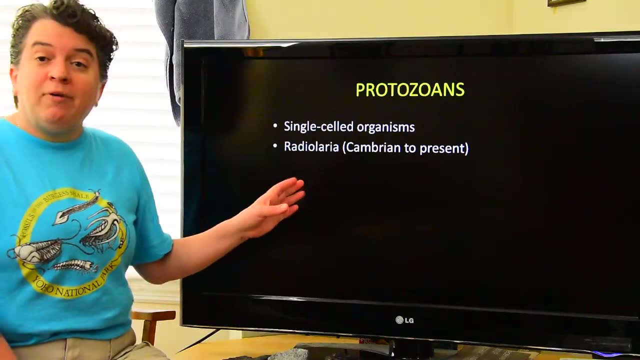 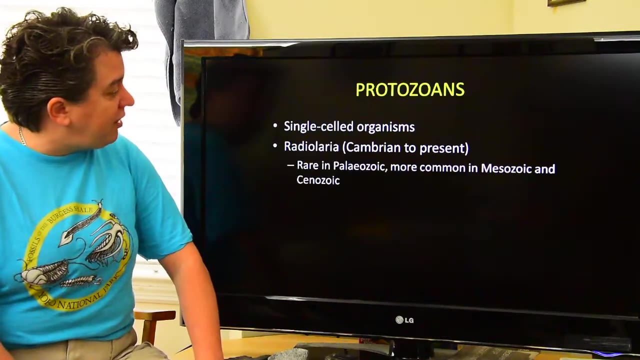 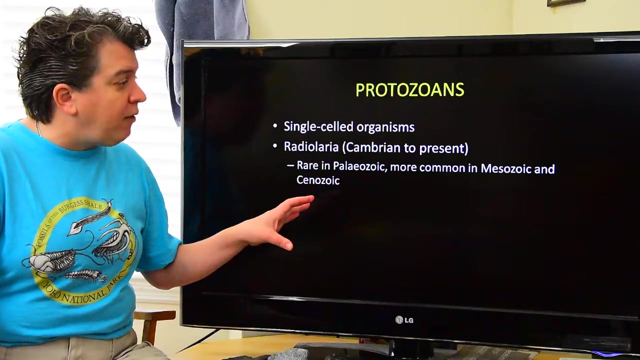 My cats are misbehaving, So hey, stop that, Joe. Alright, anyway, radiolarians also show up in the Cambrian and do still exist today, But these guys aren't really that common in the Paleozoic. While they exist in the Paleozoic, they become more abundant and more common in the Mesozoic. 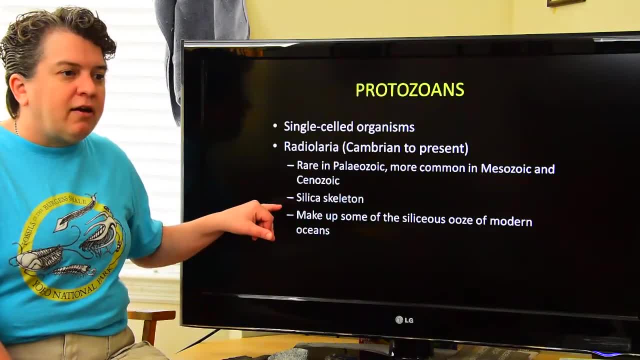 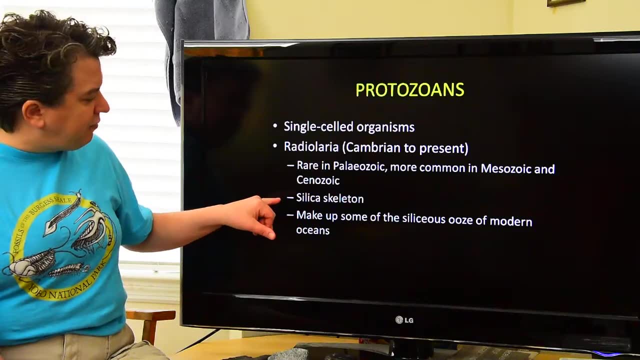 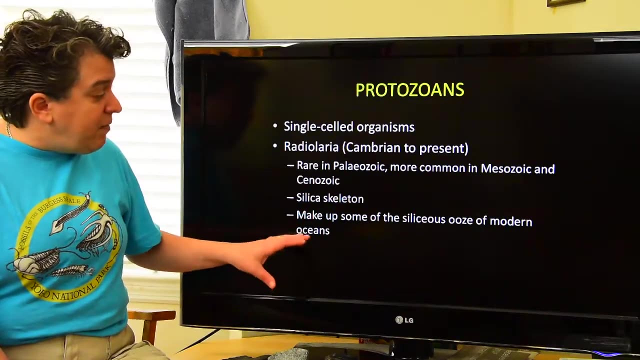 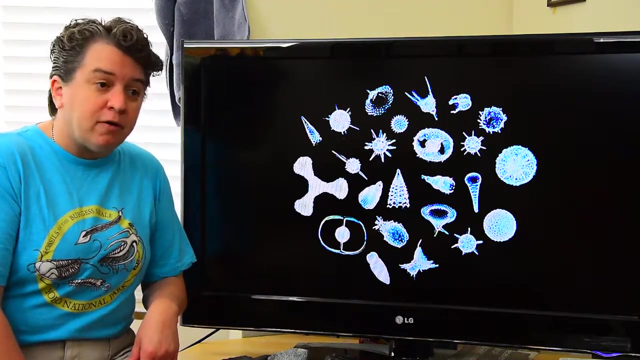 and these guys create silica skeletons. and they create silica skeletons and remember that siliceous ooze that's on the sea floor. These guys make up some of that siliceous ooze and some of them are quite pretty when you look at them underneath a microscope. 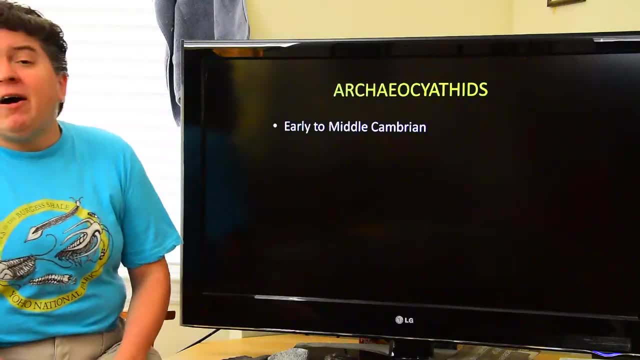 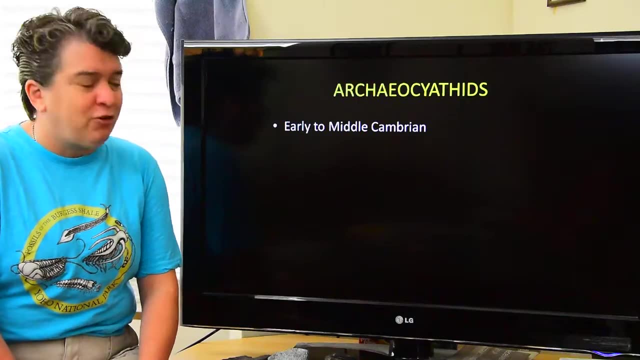 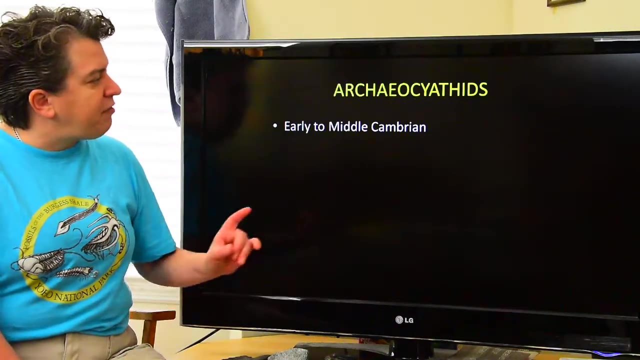 Well, I'll be honest, though I'm not that into that, I'm not that into the fossils of single-celled organisms. I think the multicellular ones are much more interesting. So let's move on to the multicellular ones. We're going to go to Archaeosciathids. 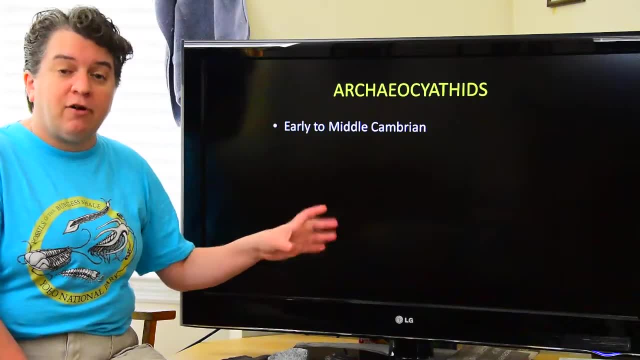 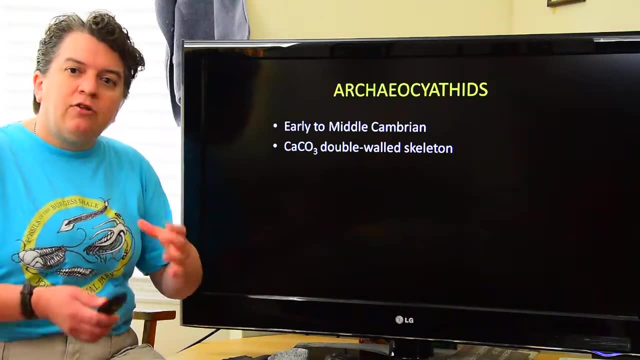 Archaeosciathids existed from the early to middle Cambrian, So these are actually an excellent index fossil And they're made from calcite and they had a double-walled skeleton to them And they're similar to the Archaeosciathids. 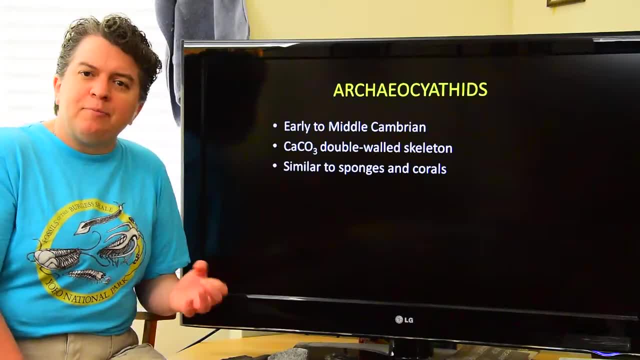 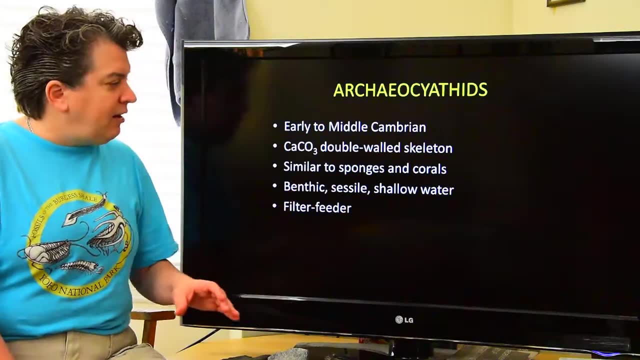 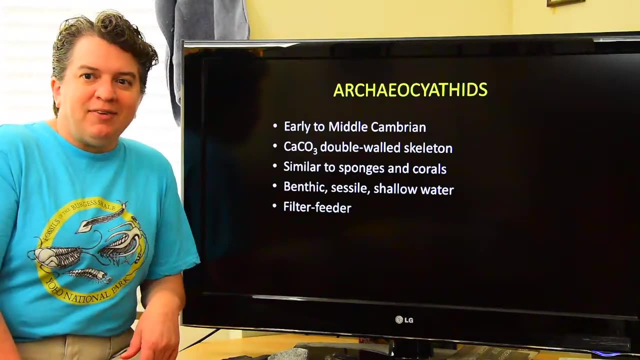 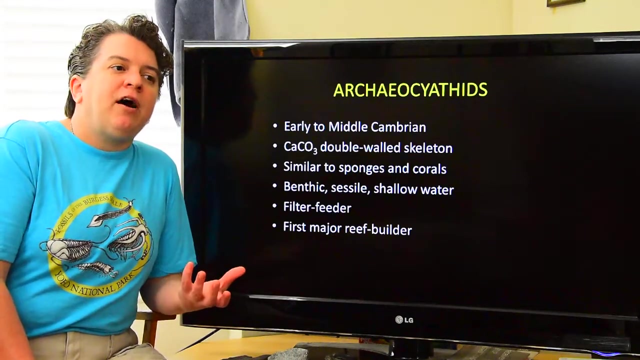 They're similar to sponges and corals, but their anatomy is different from sponges and corals: They're benthic, they're sessile and they live in shallow water. And these guys are a filter feeder. And what we're going to see also in the Paleozoic is that in every time period, reefs are being 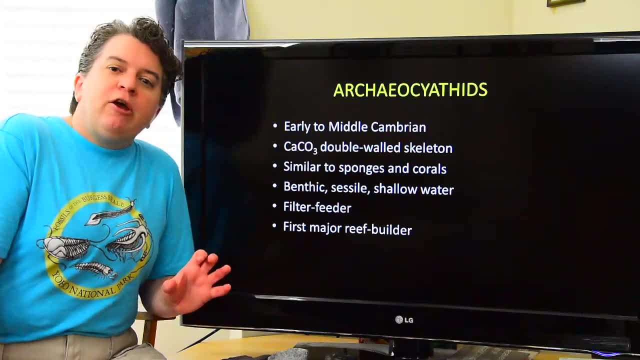 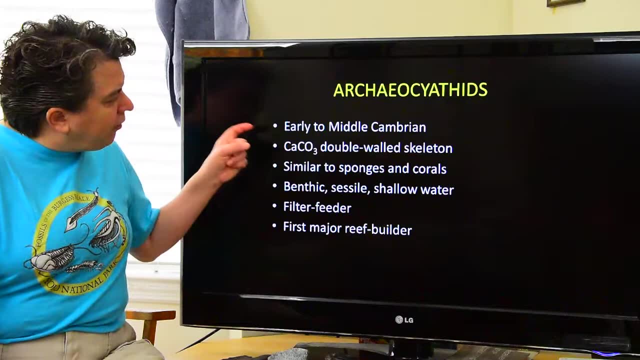 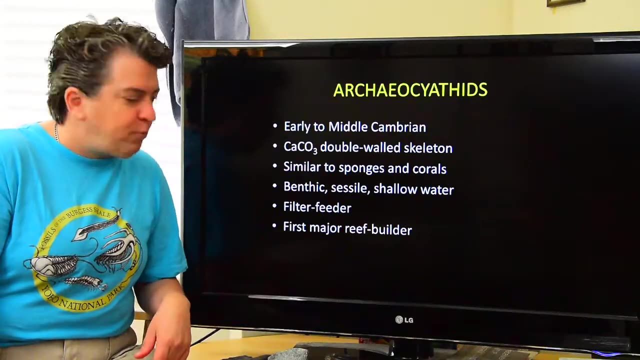 built, But it's just that. It's just that The organisms that are making the reefs differ depending on what time period we're in, And in this early to middle Cambrian, the reef builders were these Archaeosciathids, And they're our first major reef-building organism. 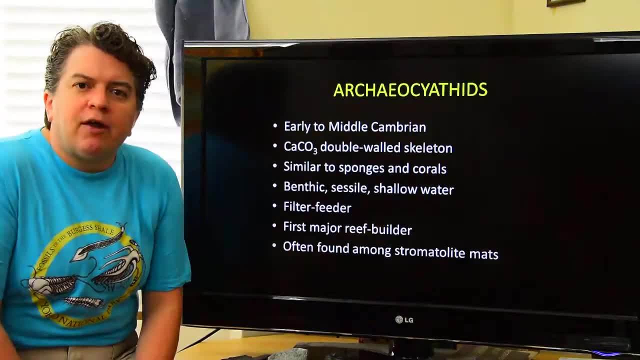 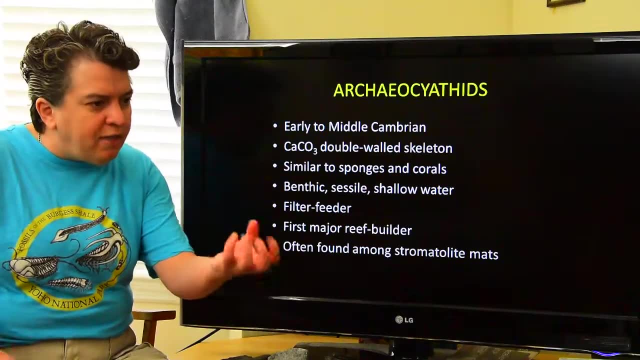 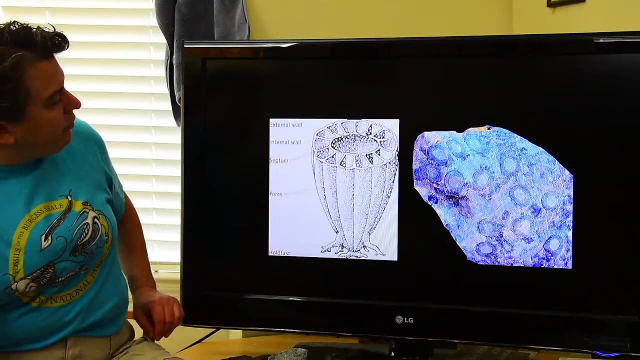 And oftentimes remember those stromatolites that I talked about, those cyanobacteria. Oftentimes you would have these mats of cyanobacteria and then interspersed among them would be these Archaeoscyathids growing up. This is what they look like. So when I talk about it, 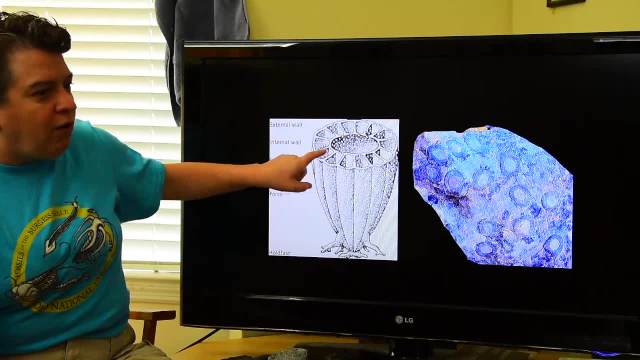 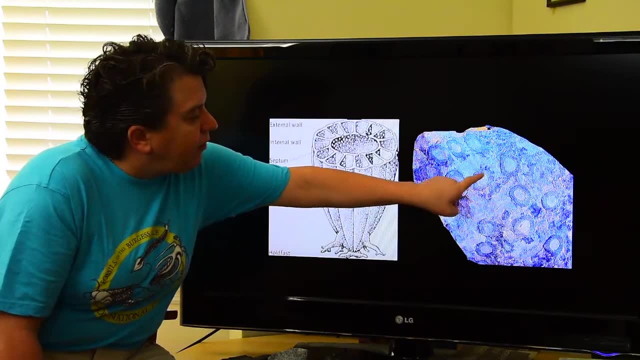 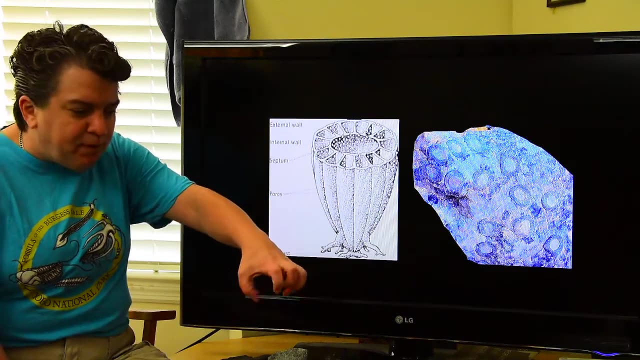 having a double wall. we have the inner wall and we have the outer wall. here And there you can see some actually preserved where there's the inner wall and outer wall And at the bottom of these these guys have this little holdfast that basically would hold it onto the sea floor. 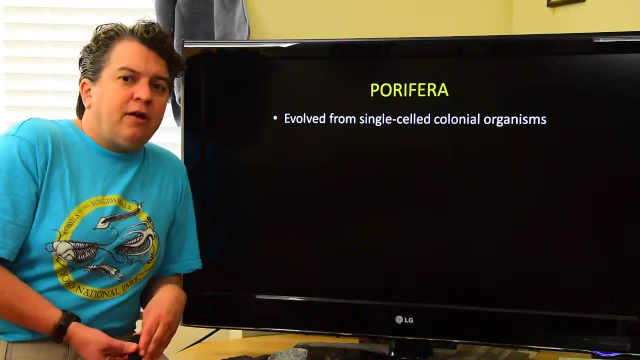 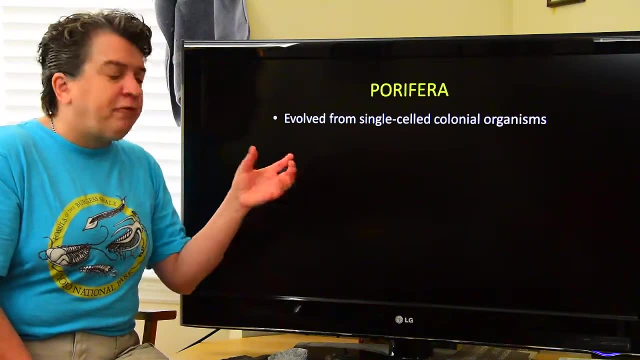 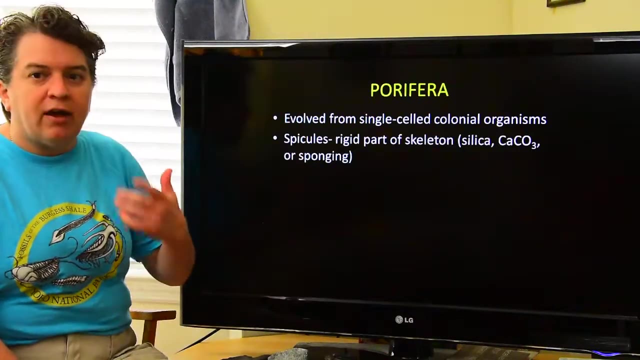 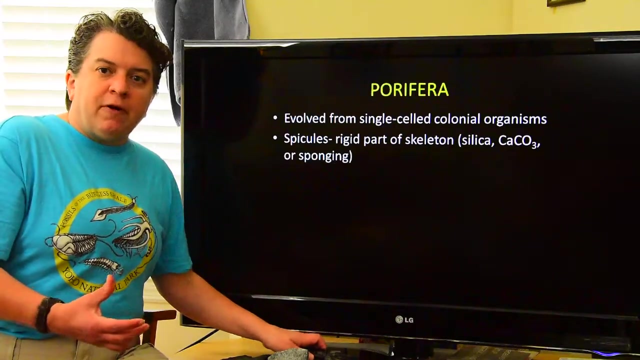 Now very similar to the Archaeoscyathids are sponges, which belong to Phylum porifera, And these evolved from single-celled colonial organisms that then basically became ultimately this multi-cellular but still very, very simple organism. Now sponges, for the most part, are very 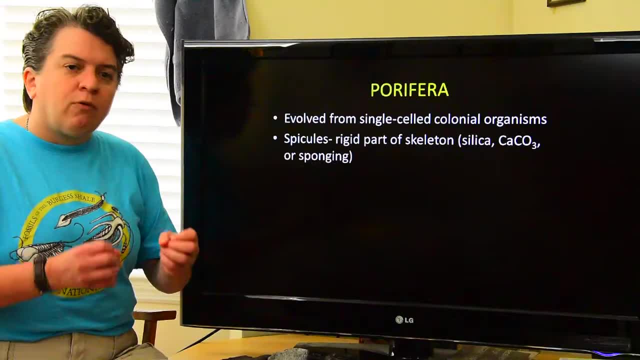 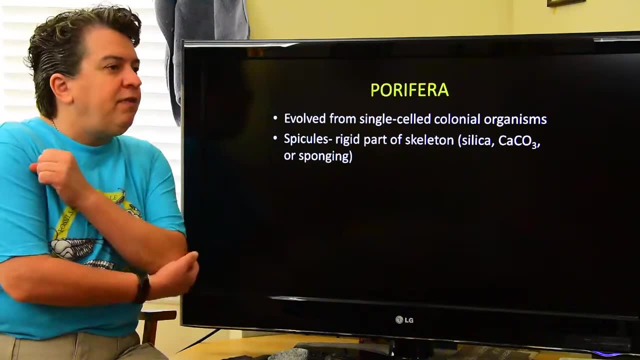 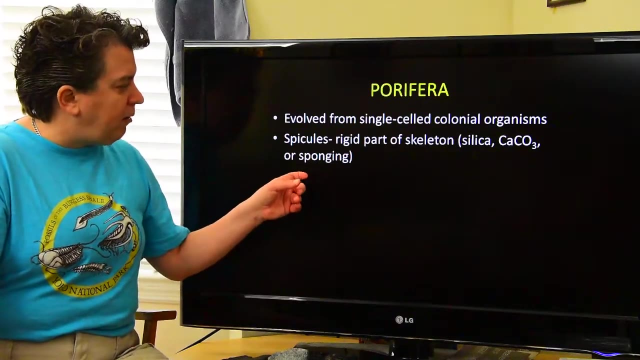 squishy and kind of soft, but they do have a rigid part to them, And we call this rigid part of them spicules, And these spicules might be made up of silica, they might be made up of calcite or they might be made up of- oops, I have a spelling error. 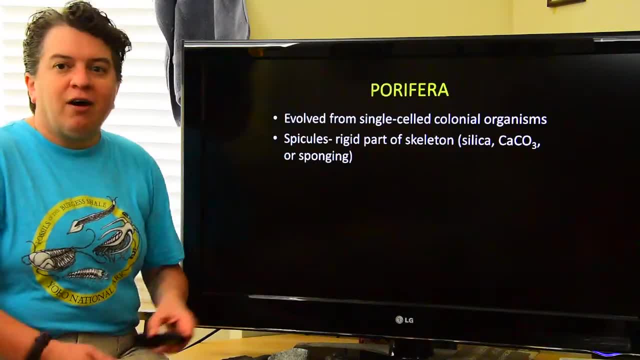 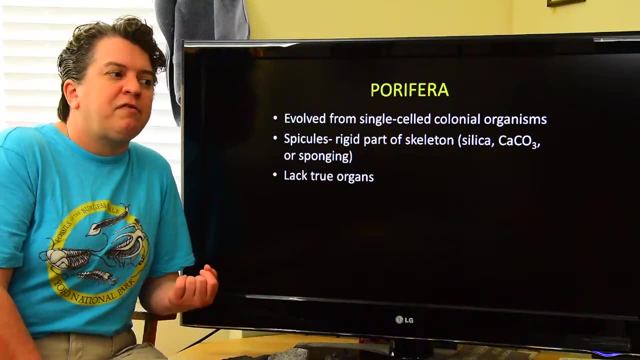 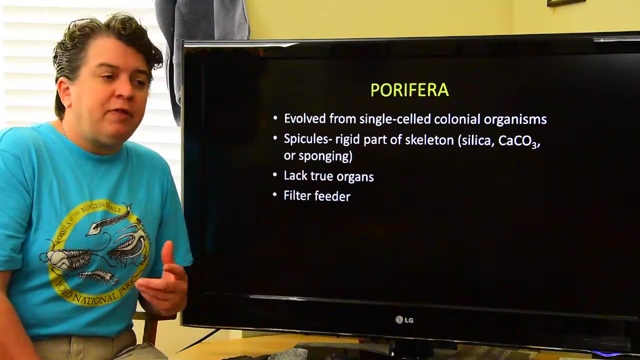 something called spongin, So take the g off that spongin, not sponging. They don't have any true organ systems, though, And so they are a very, very simple organism. They are a filter feeder. They basically eat whatever happens to be floating by. 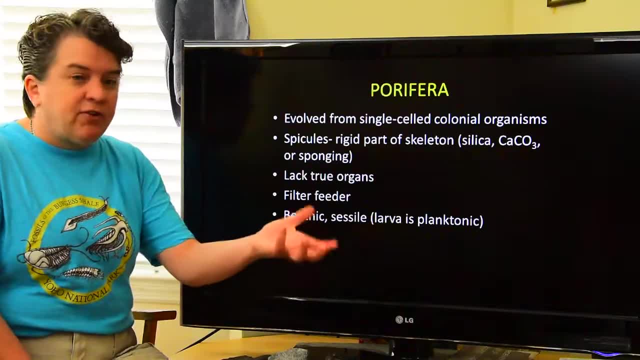 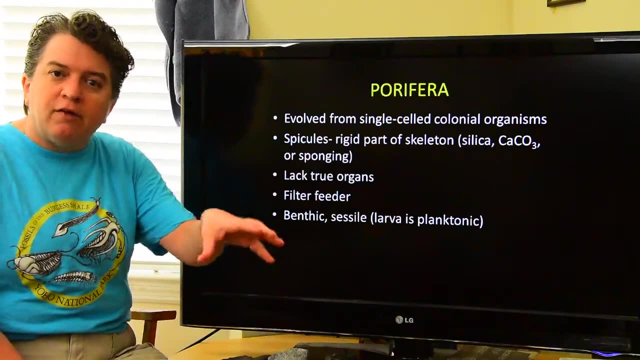 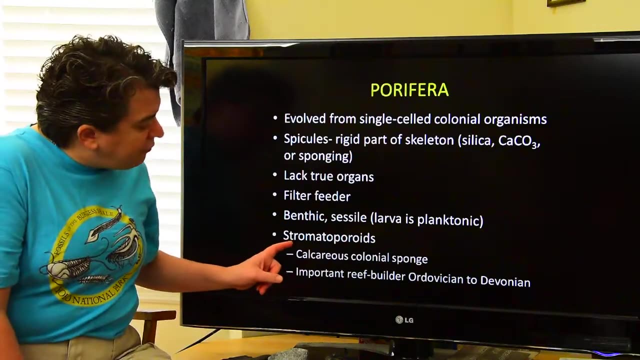 And while their larva is planktonic, their larva floats around. once we have the adult organisms, they're benthic and they're sessile. They just simply live on the sea floor. An important group of sponges in the Paleozoic are the stromatoporoids, And these were calcareous, so that's the calcite. 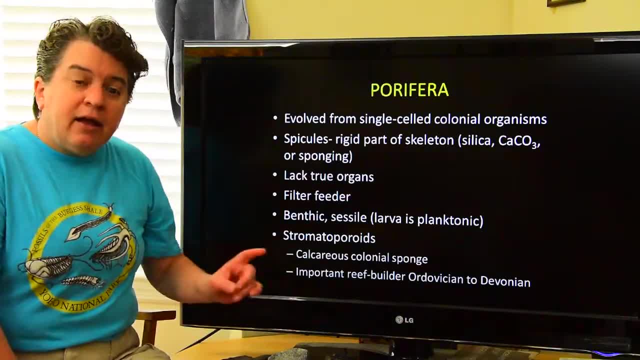 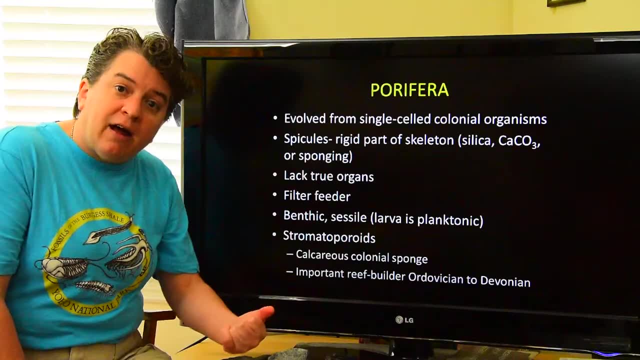 so that's the sponge. They're a colonial one And in the Ordovician to the Devonian, these guys are the important reef builder. Remember those Archaeoscyathids went extinct And this becomes the next reef building organism. 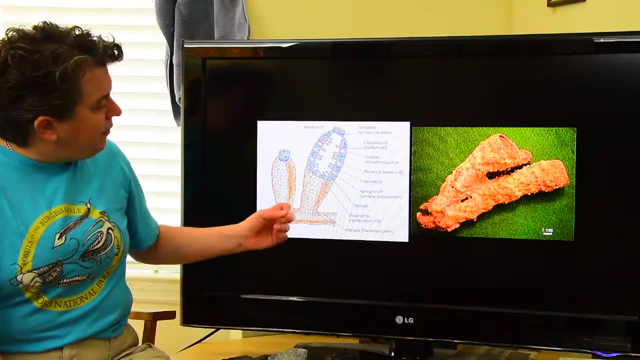 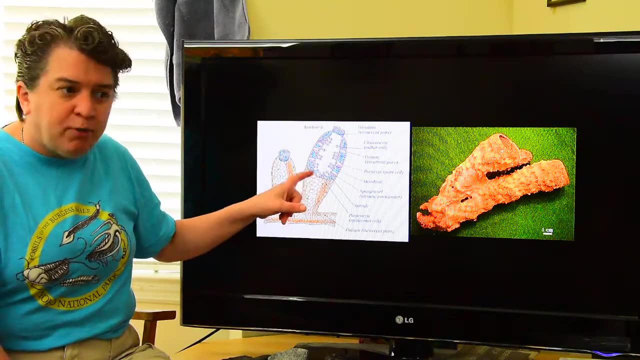 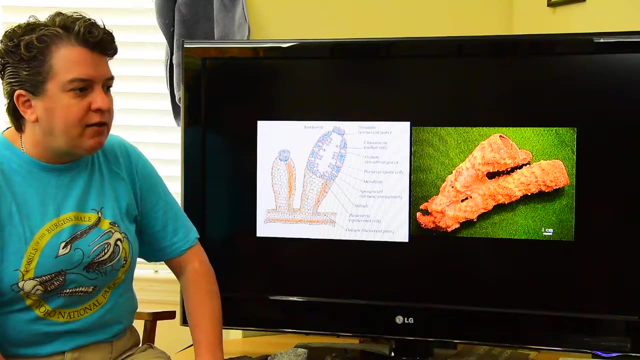 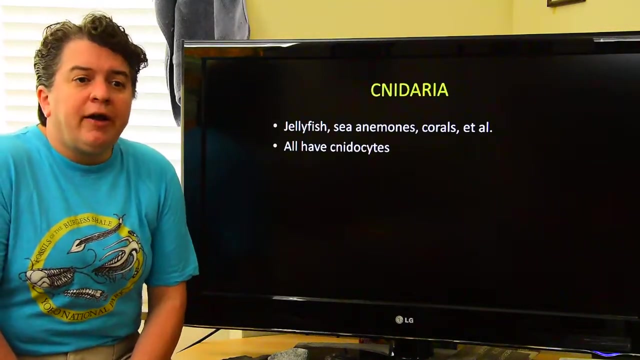 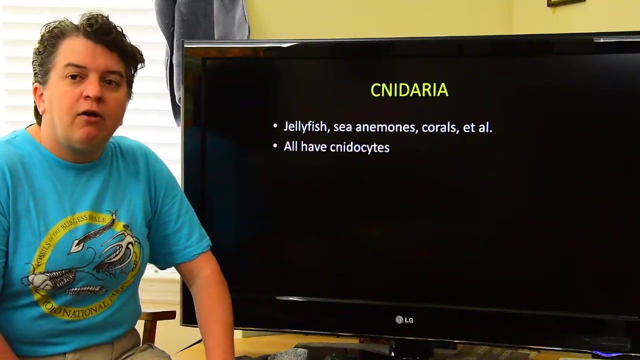 This is a typical sponge, that's a fossil of one, and this is what the sponge organism looks like. They have just this very simple structure and take in water and filter out whatever it is that they might want or might need to eat. Now, nadaria, phylum nadaria, includes jellyfish, sea anemones and corals. 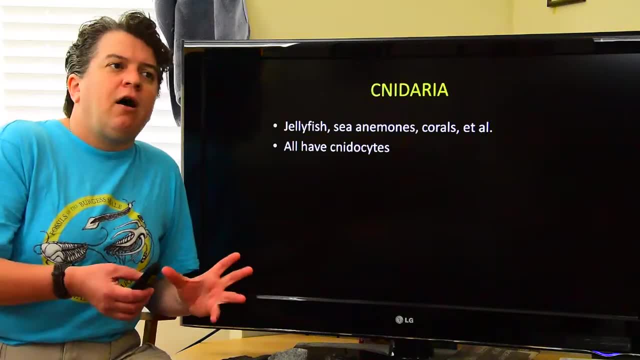 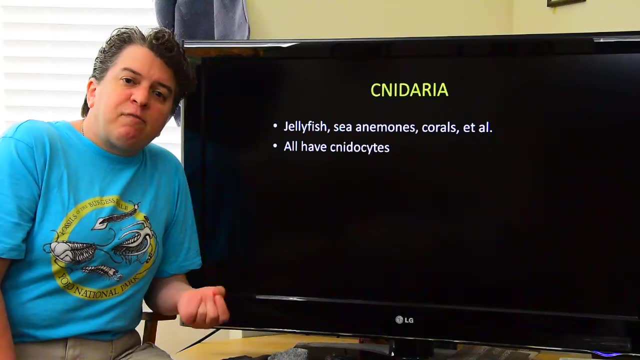 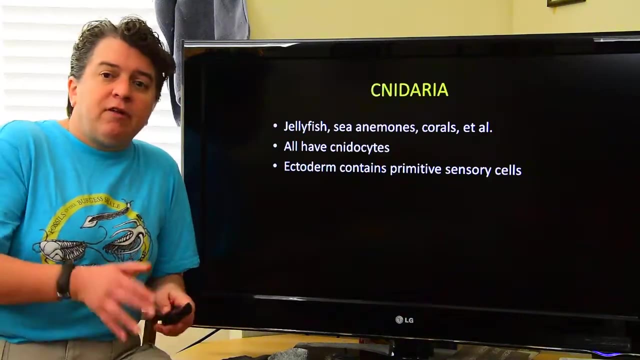 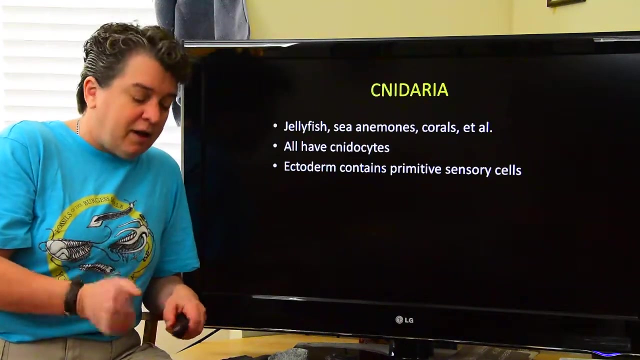 And what makes all of these similar is they have what are called cnidocytes. These are special cells that sting, And their ectoderm, that means their outermost covering, does have some primitive sensory cells in it. Now, both of these or all of these. 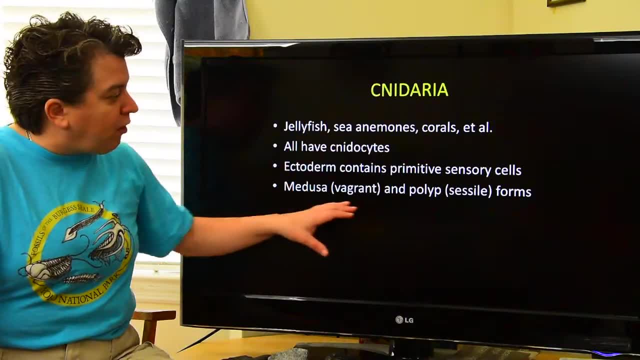 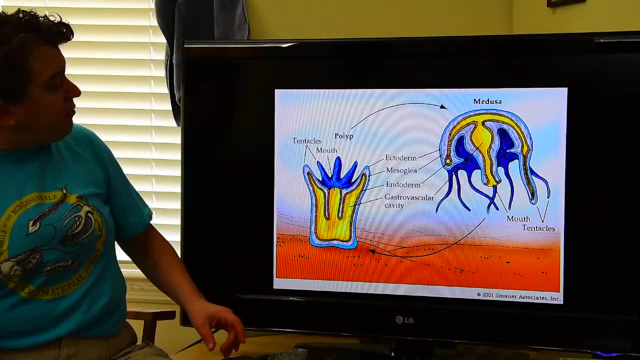 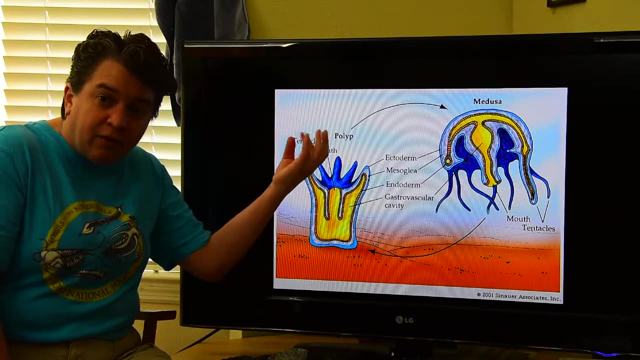 have vagrant medusa form and a polyp form that is sessile, that is stationary. So basically, the coral. if you have a coral it looks like this And if you zoom in on a coral it's going to have little tentacles. the organism. 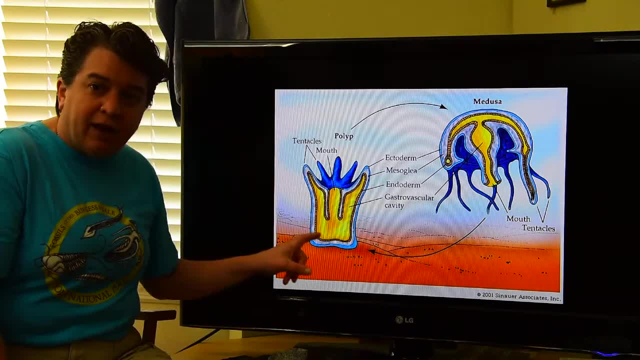 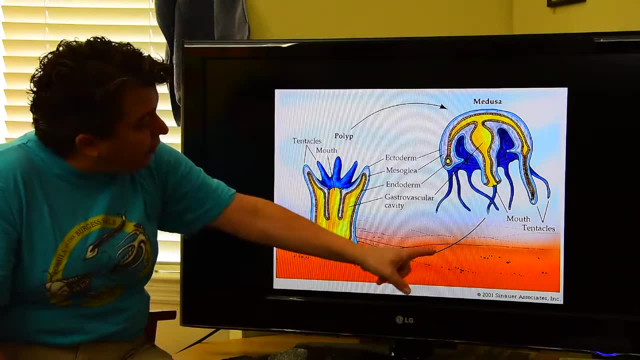 It has its mouth right there. this is its gastrovascular cavity. that's where the food goes, And a jellyfish is simply the coral kind of upside down Now. the tentacles are hanging there, but there's its mouth. there's that gastrovascular cavity. 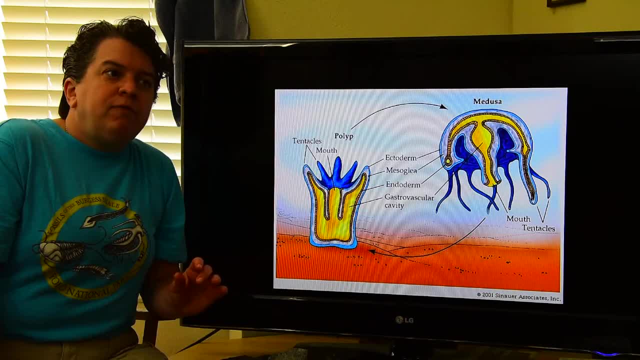 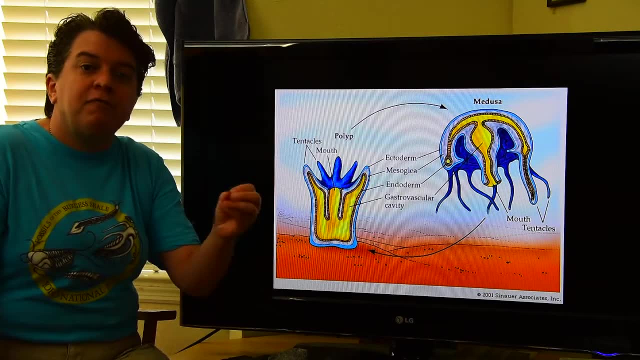 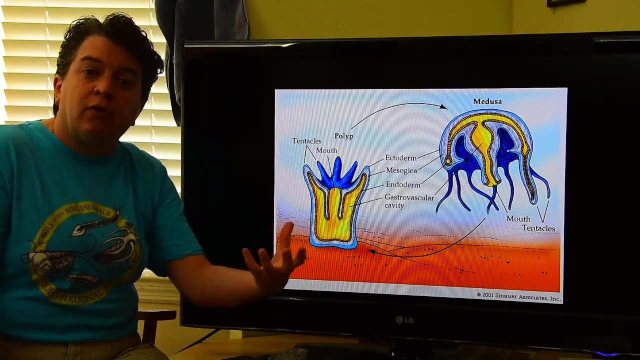 Corals. their larva stage is vagrant, it floats around kind of like the jellyfish, And then it becomes stationary and turns into a coral in its adult form. But in any case, just remember corals and jellyfish are relatives. 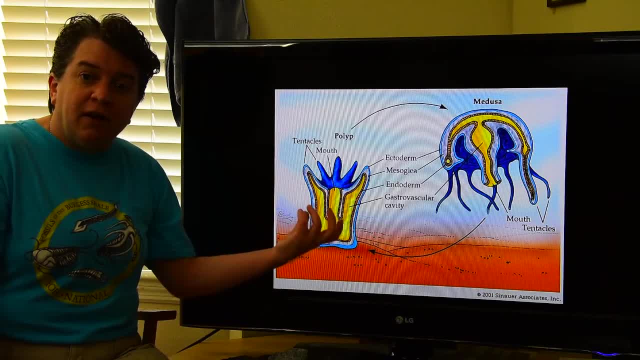 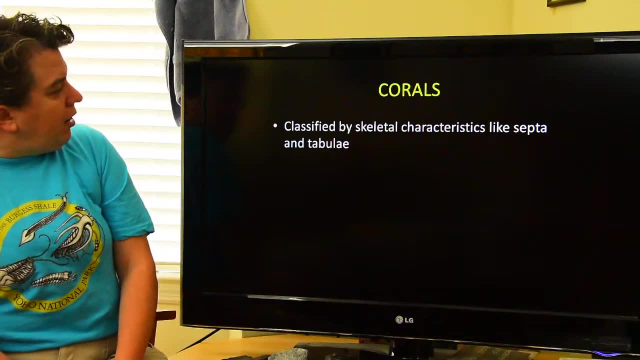 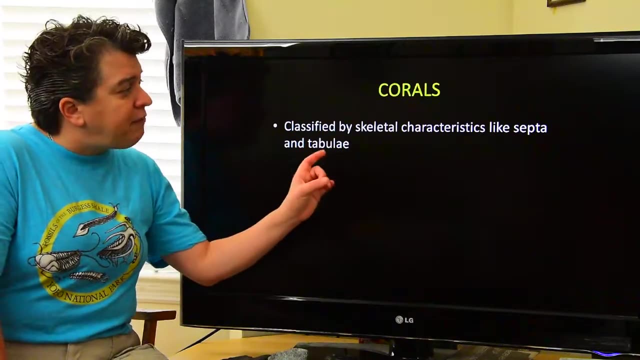 And the coral is basically just the one that sits there, whereas the jellyfish ends up moving around. Now corals are classified. there's many different types of corals that exist, And they're classified by skeletal characteristics called septa and tabulae. 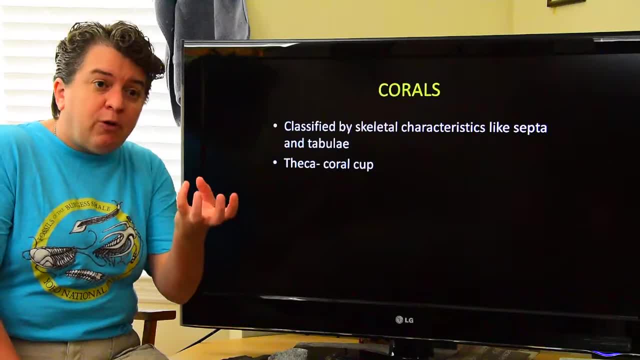 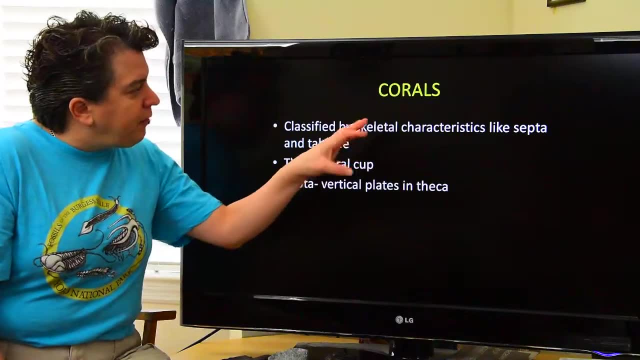 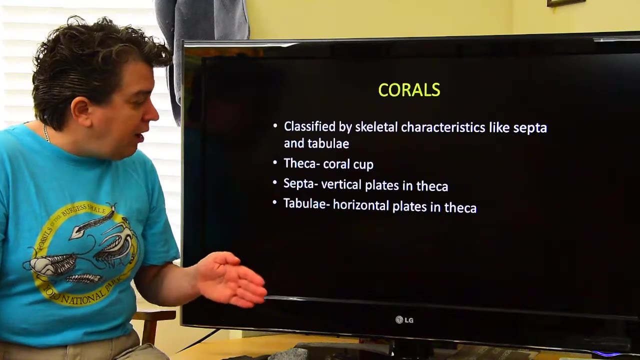 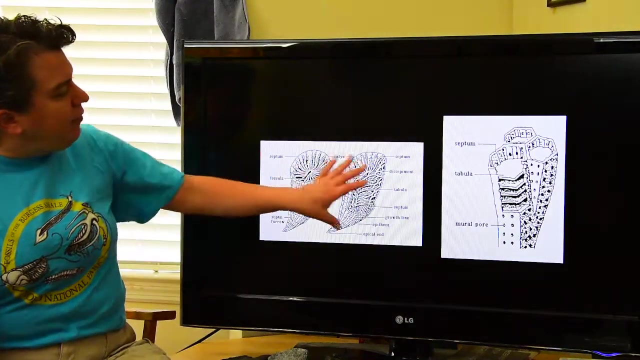 And where the actual coral organism lives is called the theca. So let's look at what these different skeletal characteristics are. The septa are vertical plates in the theca and the tabulae are horizontal plates in the theca. So if you saw in the fossil lab, you saw some of these horn corals. 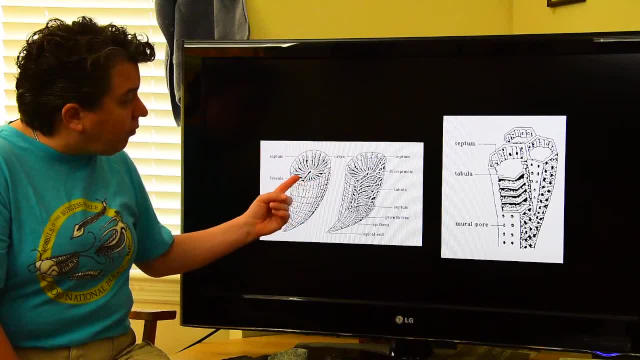 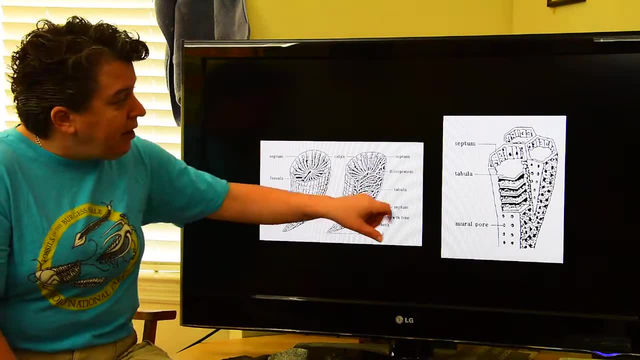 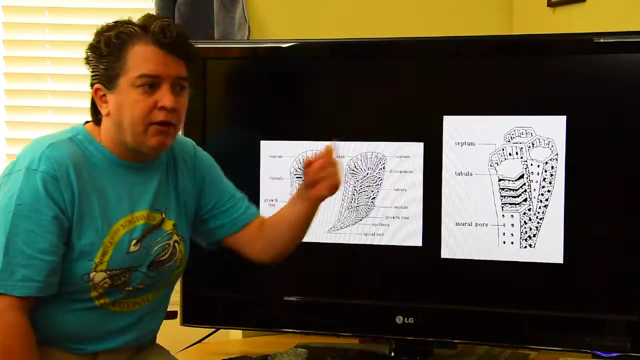 And this is where the coral organism would have lived, And so you can see septa in there and you can see tabulae in there. This is a colonial coral. Again, there's the septa and there's those horizontal tabulae. 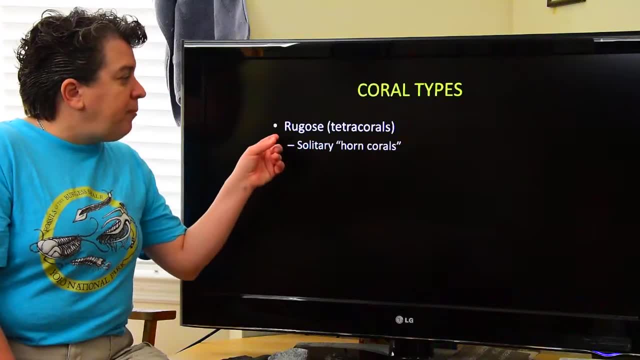 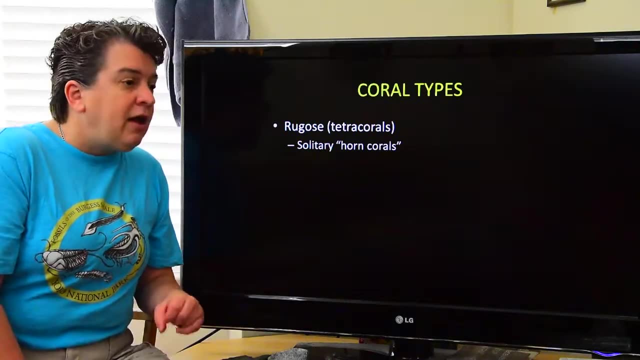 And when we look at our coral types- the horn corals that I was just mentioning- those are called rugose corals or sometimes called tetrachorals, And they were solitary, meaning there's just one coral organism in each one of these things. And the septa in them. they're called the tetrachorals because the septa added in multiples of four. These become some reef builders in the Devonian to the Carboniferous. So you're starting to see how different organisms are building reefs at different times in the Paleozoic. 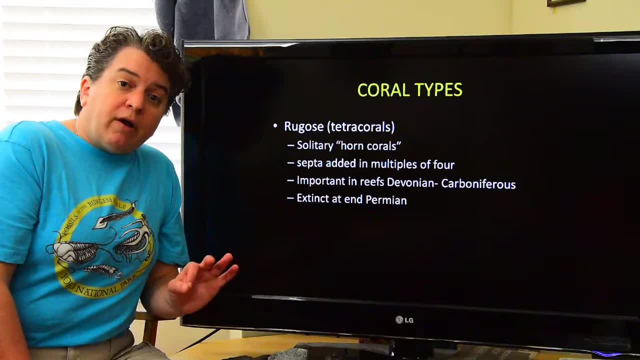 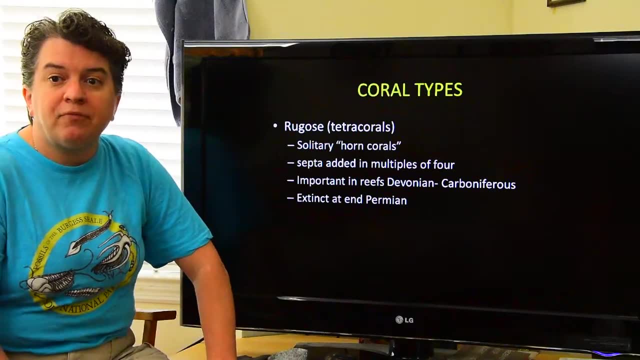 Unfortunately, rugose corals go extinct at the end of the Permian, So we no longer have this type of coral with us today. Is there a question? And this is what they. I'm sorry. I'm used to asking if there's questions. 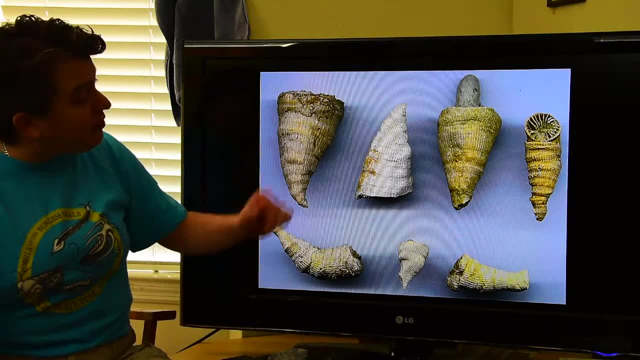 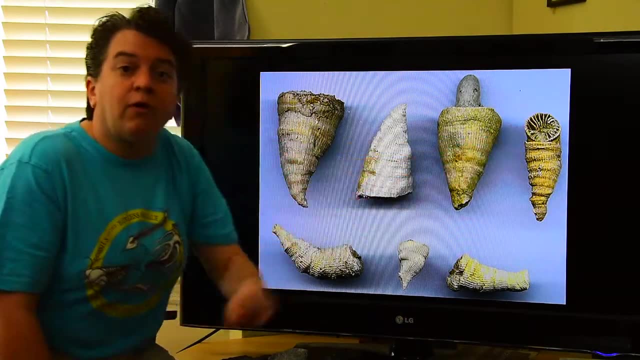 It's so strange not being able to talk to you guys, But anyway, these are some of the rugose corals. You can see why they're called horn corals, And right there that's where the little coral organism would have lived. 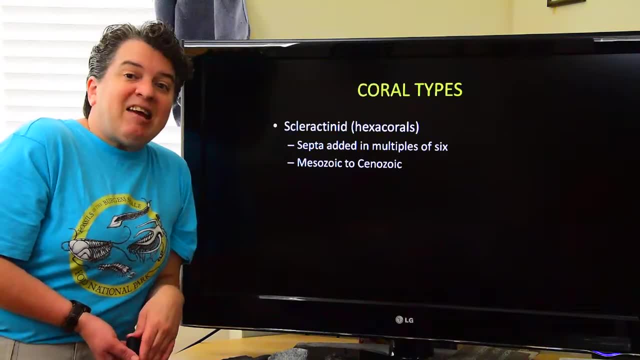 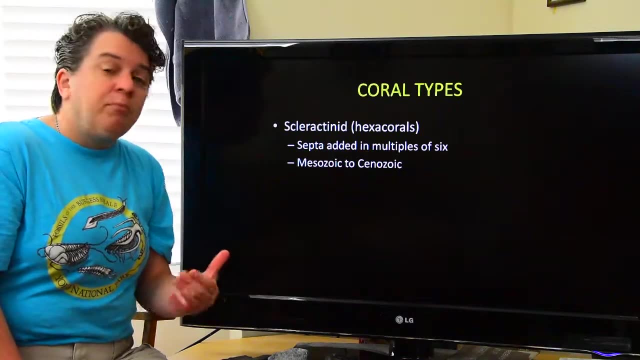 Now we also have a group of corals called scleractinid corals, or hexachorals, And hexachorals, because they're septa, are added in multiples of six. These guys are from the Mesozoic to the Cenozoic. 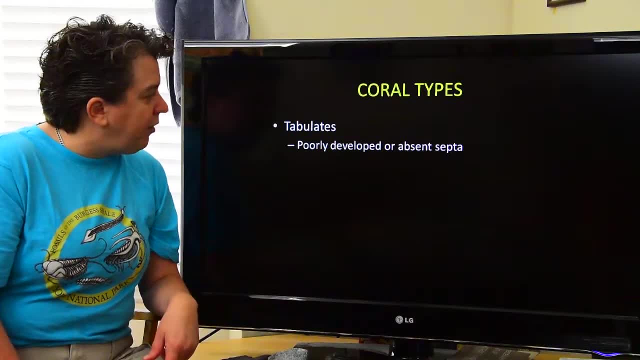 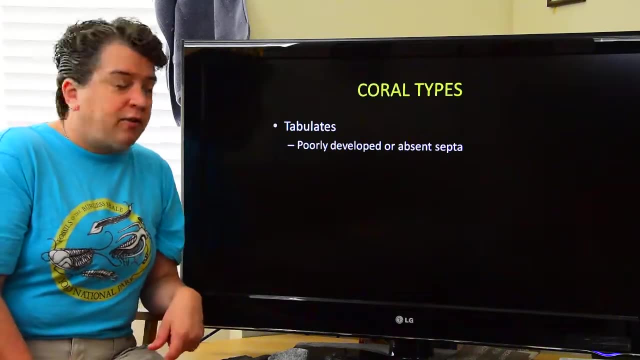 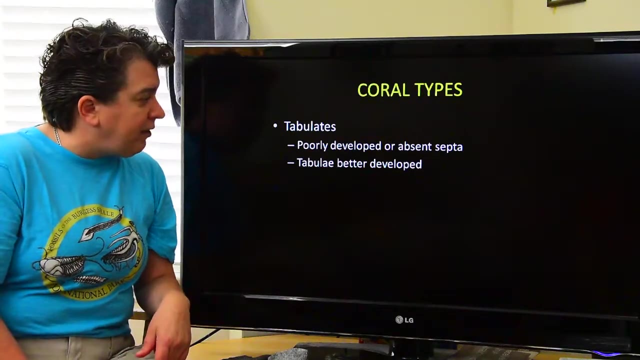 So we don't worry about these guys in the Paleozoic. In the Paleozoic, though, we do have some other corals, including the tabulate corals, And these guys don't have very well-developed septa, but they have really nicely developed tabulae. 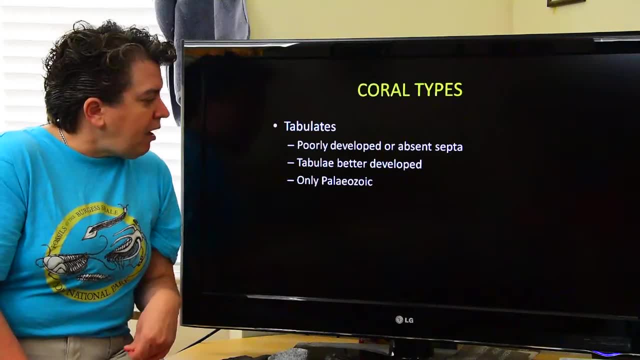 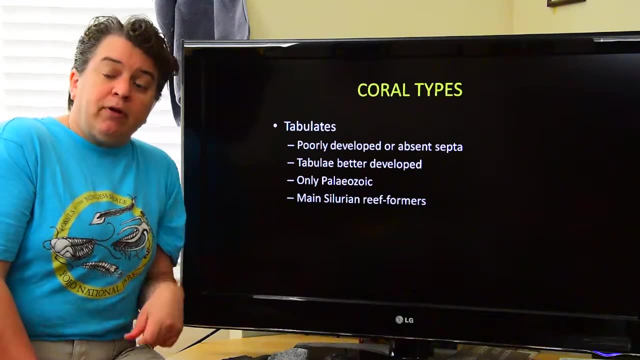 And that's why they're called tabulate corals. These only exist in the Paleozoic And in the Silurian they were building reefs. These guys are very important Silurian reef builders And this is what they look like. 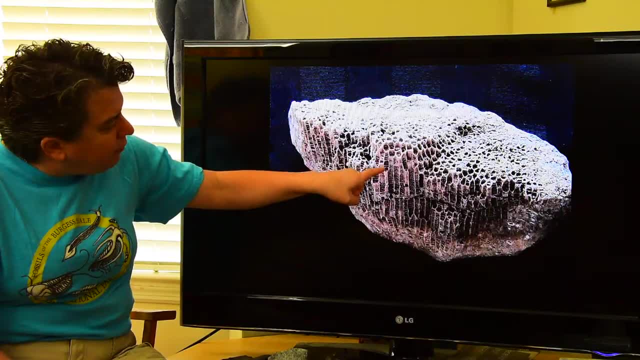 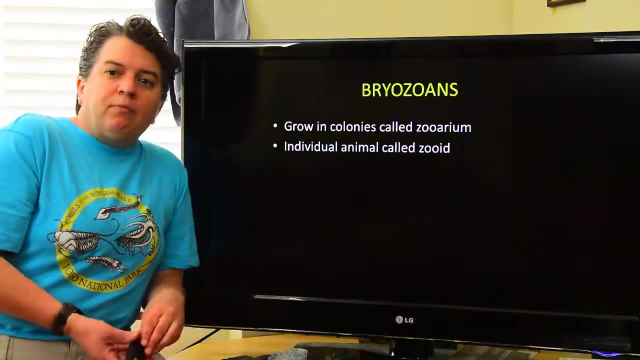 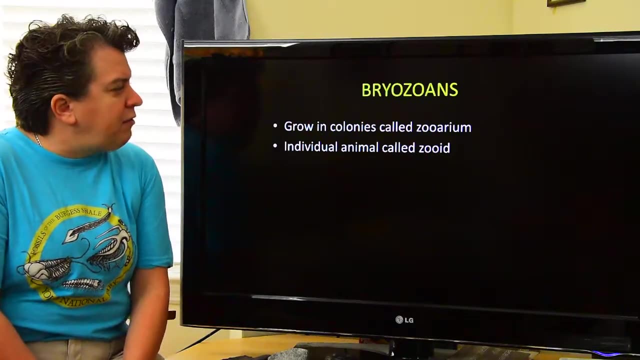 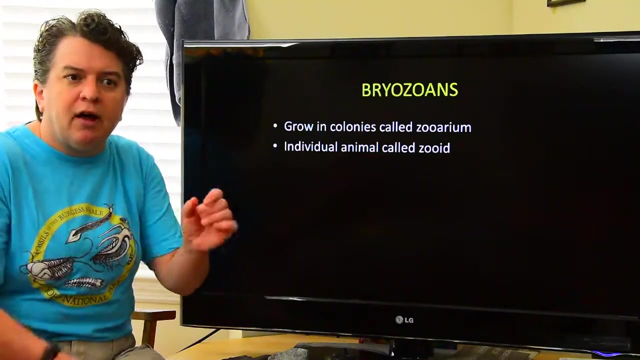 And you can see those little tabulae, those little horizontal parts to that coral in there. All right, Bryozoans. Bryozoans are a colonial animal that is similar to a coral. They kind of live in these colonies All together.